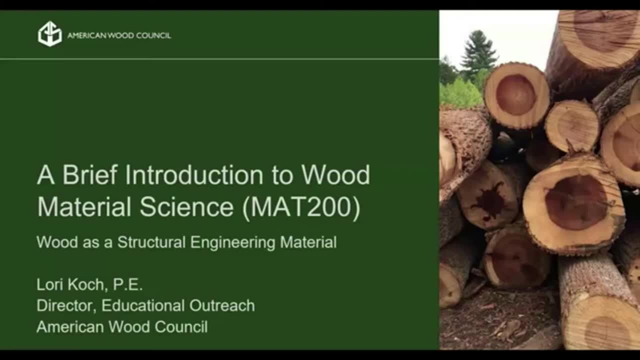 Hello everyone and welcome to today's presentation. a brief introduction to wood material science. My name is Marci Weber and I'll be your education team moderator for today's presentation. Today's webinar is going to run one hour. This means that you must be present for 54 minutes of. 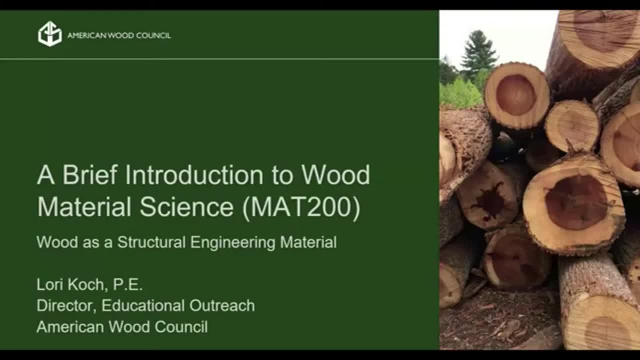 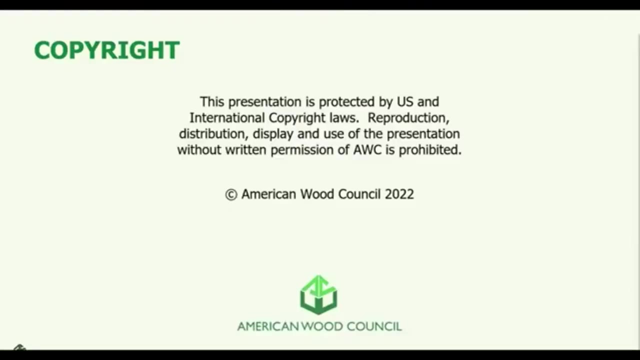 the 60-minute webinar in order to qualify for continuing education credit. Please stay on for the live question and answer session at the end to ensure that you meet the time requirement. Today's speaker is our Director of Educational Outreach, Lori Cook. This course is copyrighted and not eligible for reproduction. 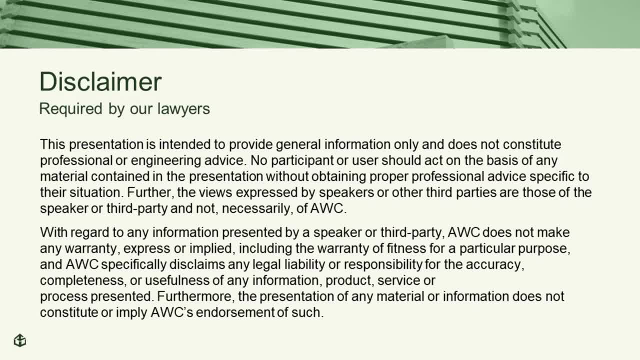 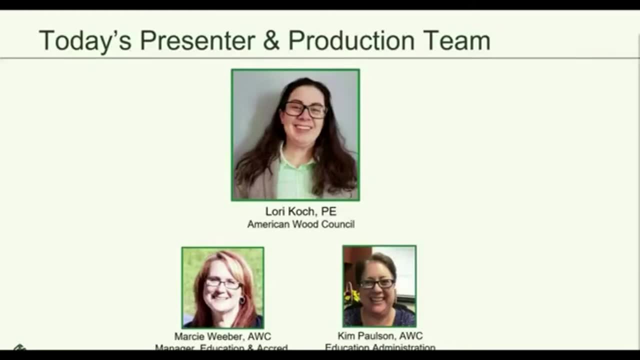 And here we have just a quick disclaimer. Please note that this webinar and associated slides should not be used as a substitute for competent engineering support and expertise. And here's our team that's providing the course for you today. Again, our speaker today is Lori Cook, Director of Educational Outreach, Lori Cook. 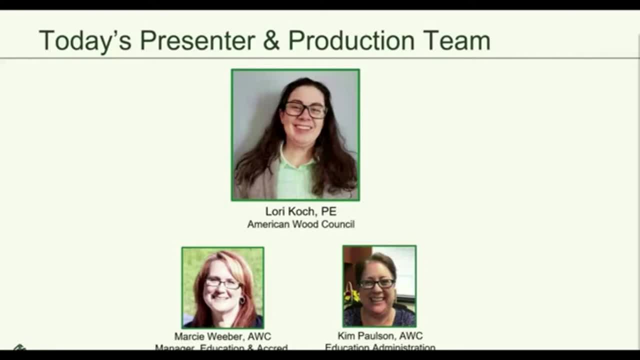 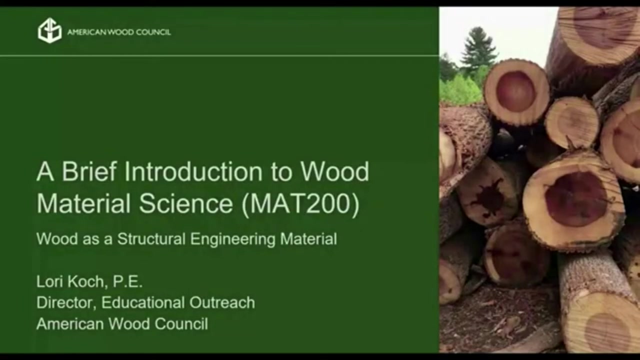 And behind the scenes is myself, Manager of Education and Accreditation, Marci Weber, and our Education Administrator, Kim Paulson. Now let me give you over to Lori to discuss material science. All right, Thank you, Marci. Thanks everyone for joining us today. My name's Lori Cook. I'm the Director of Education and Accreditation. 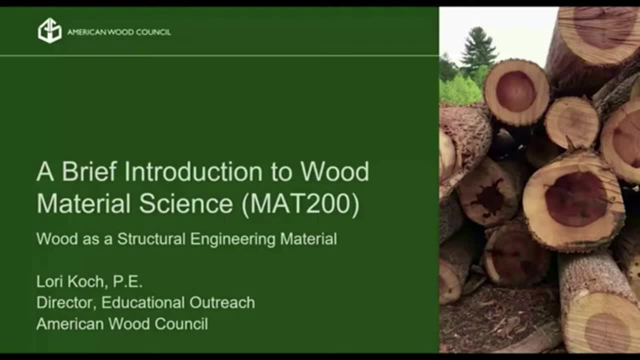 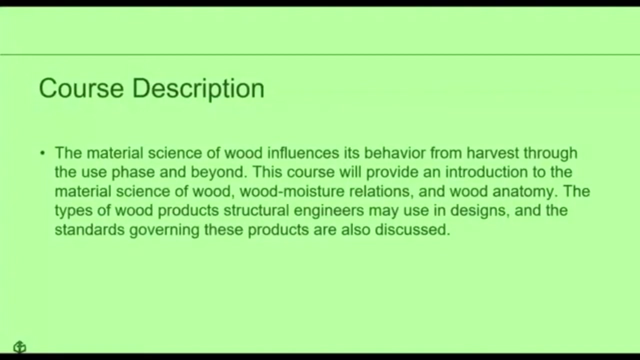 I'm the Director of Educational Outreach with the American Wood Council And today we're going to talk about a brief introduction to wood material science. So we're going to explore some of the finer points of wood as a structural engineering material from the material science standpoint. Our course description is here, I'm going to assume. 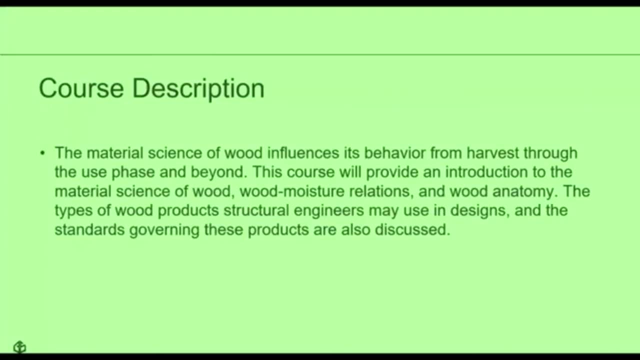 most of you saw it when you signed up for the class. The genesis of this class is that you know most of us, as structural engineers will get a class, at least one lecture, during our undergraduate careers, where we learn about a little bit about the material science of wood, But a lot of us don't really. 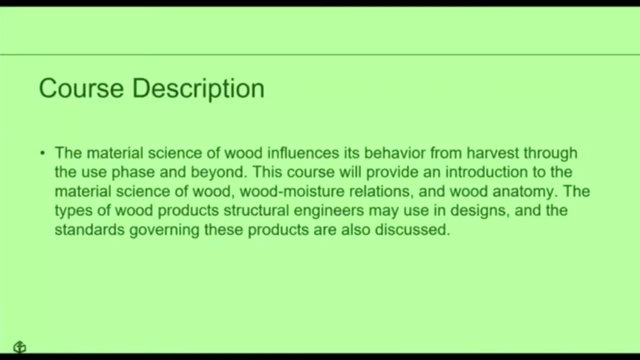 get a refresher on that or might not spend a lot of time dealing with that, And these are certainly elements of the material that can impact how you use it when you design. So I thought it would be a good opportunity for us to spend a little bit of time this month talking about the material science. 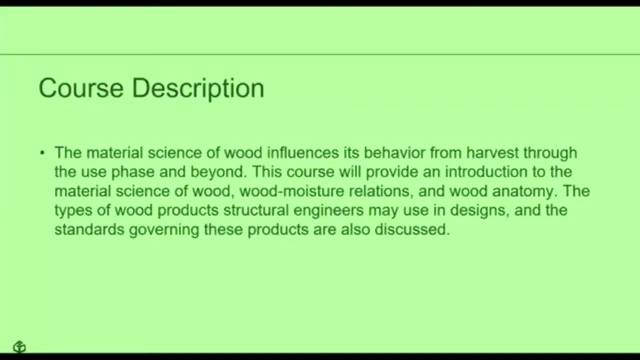 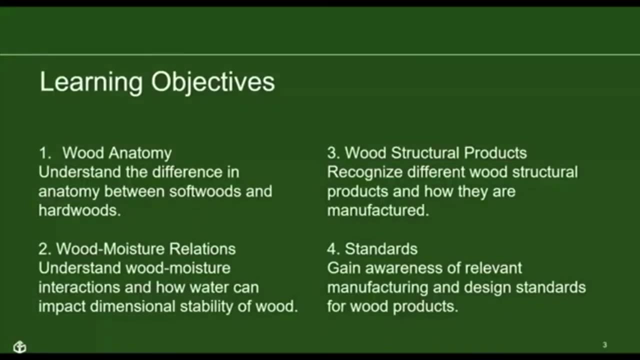 of wood and some of the points that we would, as structural engineers, want to pay attention to. Our learning objectives are here as well. These were also presented when you signed up for the course, so I won't linger on these too long. 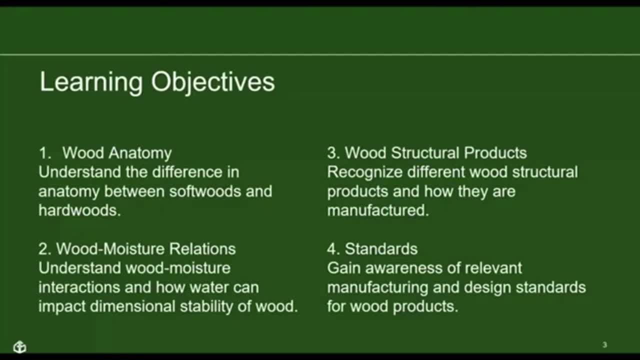 We'll spend some time on the anatomy of wood and talking about the difference between softwoods and hardwoods. We'll discuss wood moisture relations right and how water can impact the dimensional stability of wood. We'll talk about some of the different wood structural products that you might encounter as a structural engineer And we'll talk about 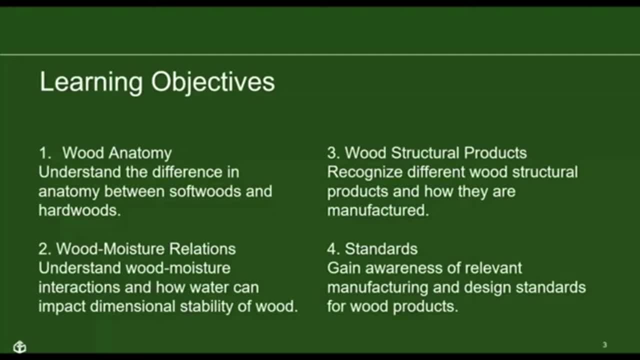 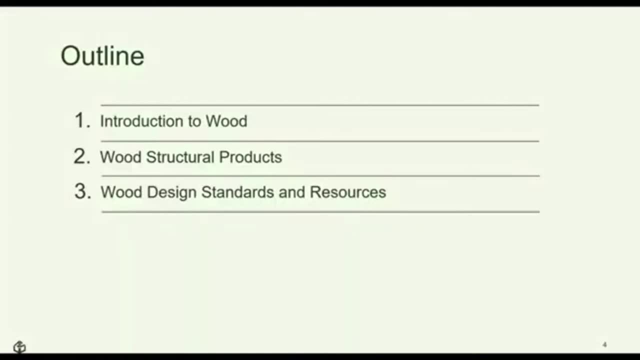 some of the standards that are important when using some of these wood products as well. So a brief outline for today. I'll just give you an introduction to wood: what it is and how, how we classify different elements of wood. Then we'll go into talking about some different. 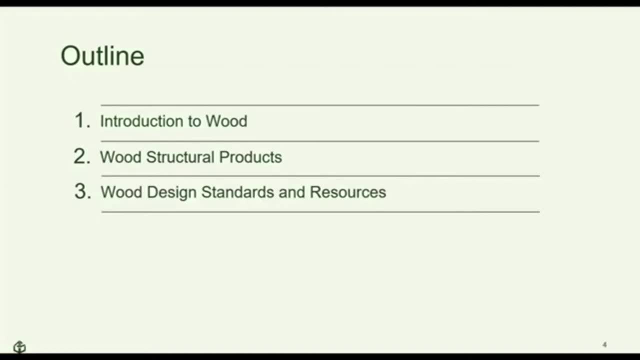 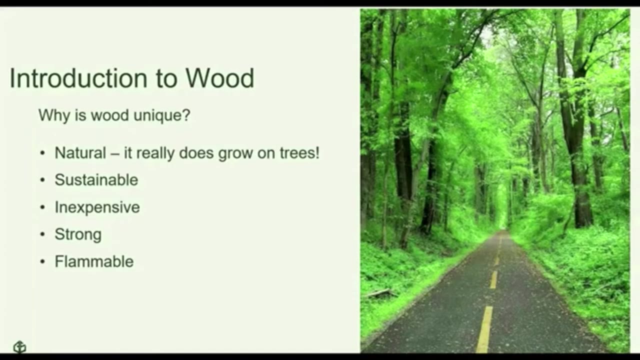 wood structural products And finally, we'll close it out with some wood design standards and resources before we get into the question and answer portion of the program. So our introduction to wood. So why is wood unique? It's unique for quite a few reasons. 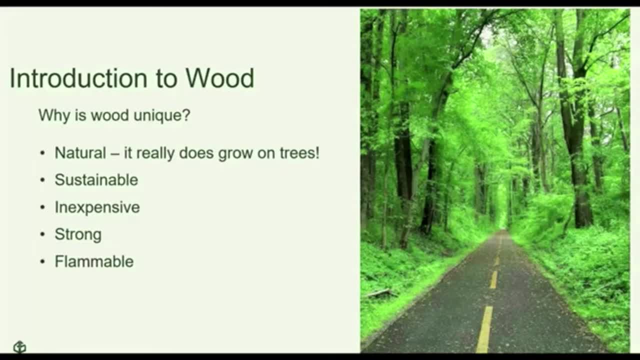 beyond even what I've got listed here, but it is a natural product. It really does grow on trees. It's sustainable. So we have harvest cycles of 30 to 50 years. We can cut down a tree. We'll typically plant more than we cut down as part of our working forests, which we'll talk a little bit. 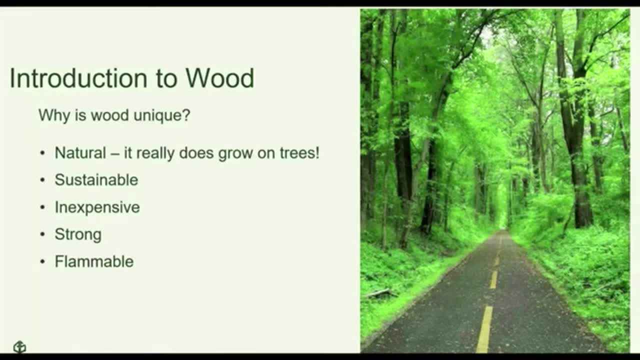 more about. It's relatively inexpensive. It has a very high strength to weight ratio, So it's a very strong material, given how light it is, And it's flammable. So that is something that that we do need to be aware of when we're designing structures made of wood. 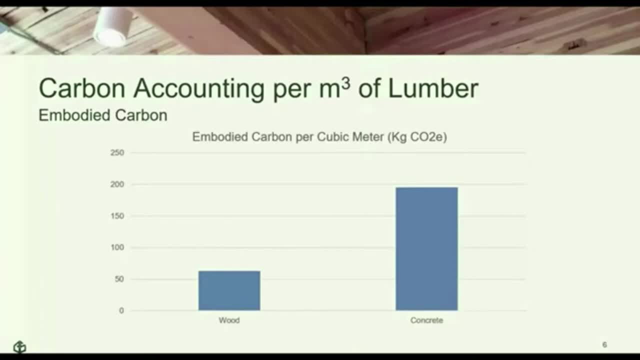 When we look at the carbon accounting of lumber, there is a lot less embodied carbon in wood than there is in other structural materials. Wood is one of the only materials that actually absorbs carbon from the atmosphere as it grows And when we put that wood into a building product and then put it in a building. 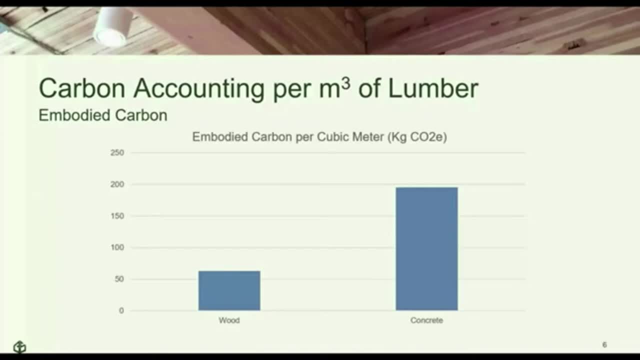 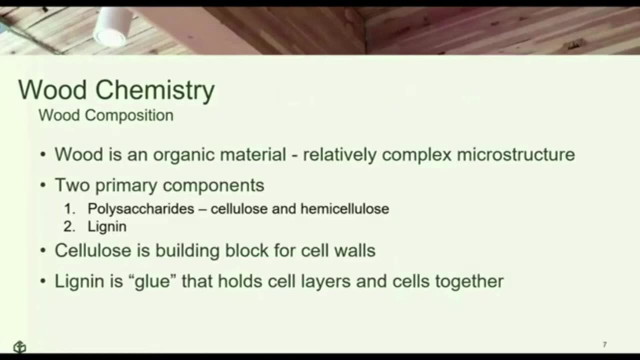 that carbon is locked away for the life of that product for its use. Dr Leisha Young, The chemistry of wood is is very interesting and there's several branches of wood science devoted to different elements of wood chemistry. so to to get into that all today, we would we need many more hours than we have to. 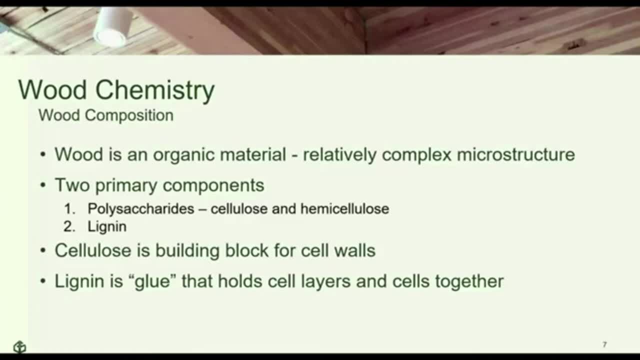 together, but suffice to say that wood's an organic material with a relatively complex microstructure. it's got two primary components, polysaccharides, which are cellulose and hemicellulose and lignin. and cellulose is the building block for the cell walls and cellulose is a a linear polymer of. 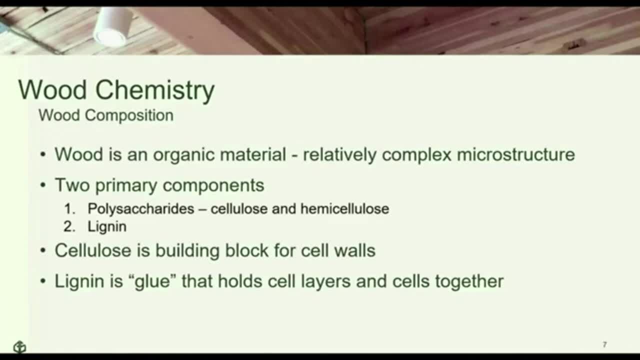 glucose units and the degree of polymerization, for for that molecule can uh range from, you know, 15 glucose units to many thousands of them glucose units. so it's a it can be a very long chain polymer. lignin is is the glue that holds the cell layers and the cells together, and this is a three-dimensional polymer with no 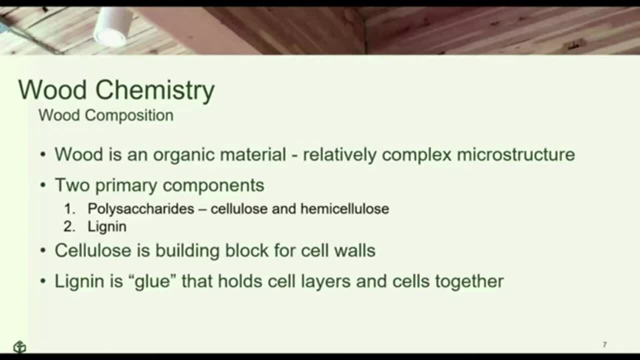 ordered arrangement it's. it's kind of amorphous, and understanding the components of wood is important because this can help you understand decay. we have different, different critters that that eat different parts of the wood. so it's if you're investigating a failure where you've seen decay or or evidence of insects, you know it's. it's good. 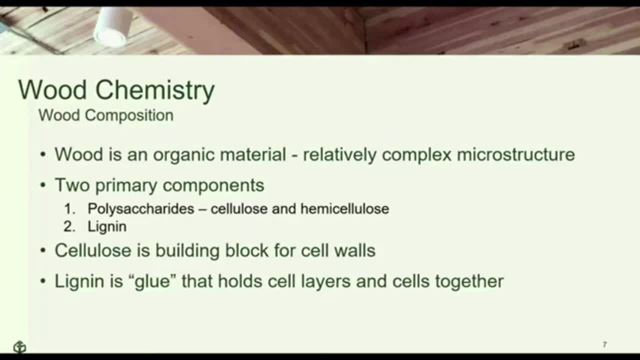 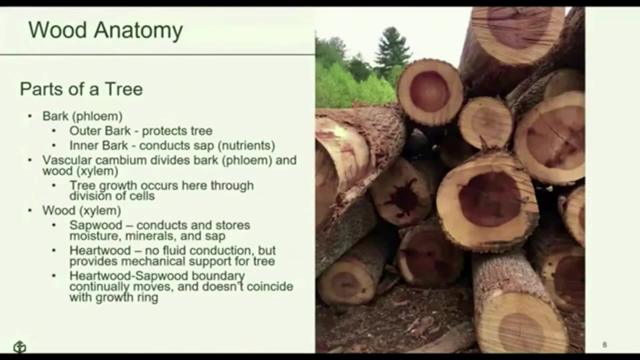 to know that brown rot, for example, or dry rot uh will talk target the cellulose uh, as will termites. termites like to eat the cellulose uh, whereas white rot will target the lignin as far as the parts of the tree. we have three main elements of the anatomy that we 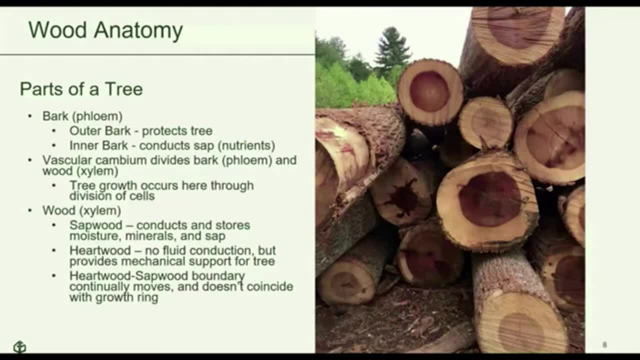 discuss. when talking about wood, we have the bark, also known as the phloem, and that's further divided into the outer bark and the inner bark. the outer bark is used to protect the tree. the inner bark is where we have sap, which is the, the water and nutrients, uh, that that feeds the tree. 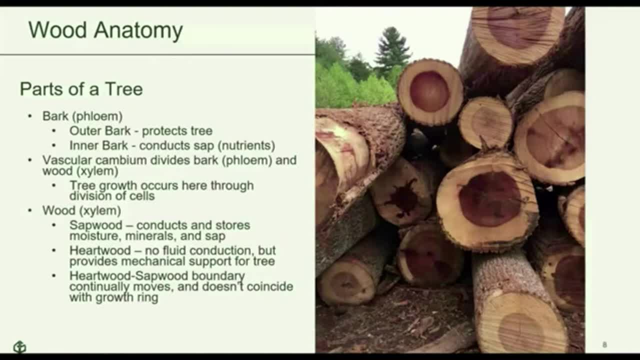 is conducted in the inner bark. In between the inner bark and the wood we have a one cell thick layer called the vascular cambium, and this is what divides the bark, or the phloem, from the wood or the xylem, and this is where the tree growth occurs through division of cells. So some of those cells- 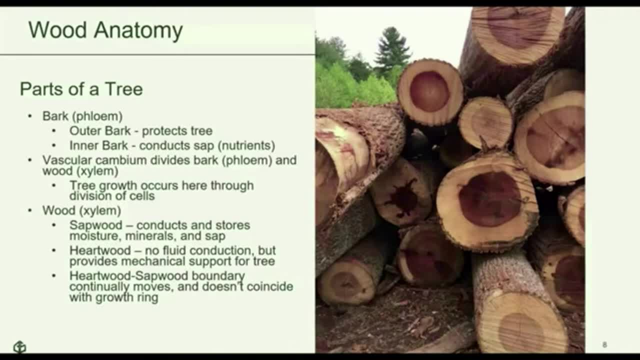 will move towards the bark and become bark cells. Some of those cells will move towards the wood and become wood cells, Getting into the, the wood or the xylem. we have two elements of that as well: that we described The sapwood, which is the outermost or and the youngest portion of the wood. 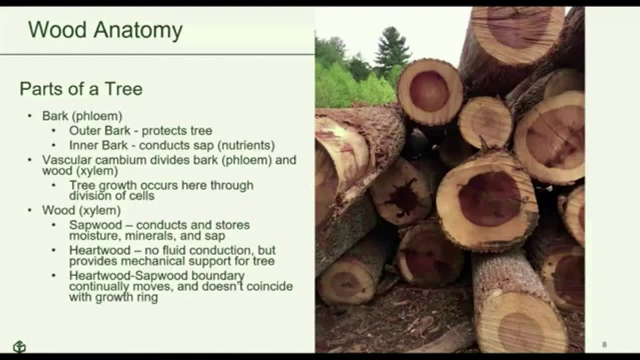 that would be the wood that is closest to the vascular cambium And the growth boundary, and we have the heartwood, which is closer to the center of the tree. The sapwood is, as you might guess, used for conduction and storage of sap moisture minerals. 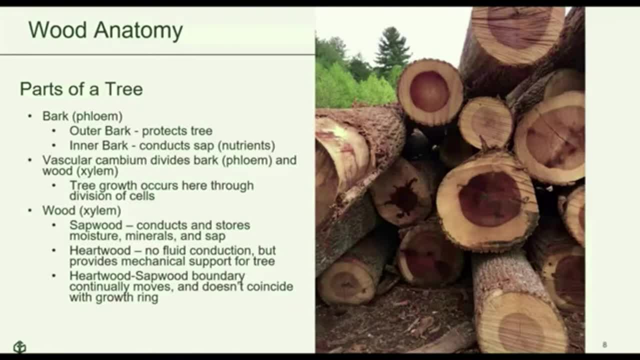 and the heartwood is in the center of the tree. It's not providing any sort of fluid conduction but it does provide mechanical support for the tree And the heartwood sapwood boundary is moving continually throughout the life of the tree and it doesn't necessarily coincide with any. 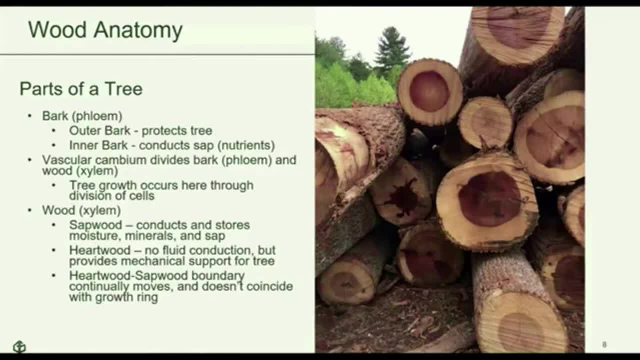 growth rings or or anything like that. and in this photograph you you see here this i- i took it a lumber mill a few years ago- some interesting expressions of the heartwood sapwood boundary. so in some of these logs, uh, you know the the heartwood sapwood boundary is kind of round. 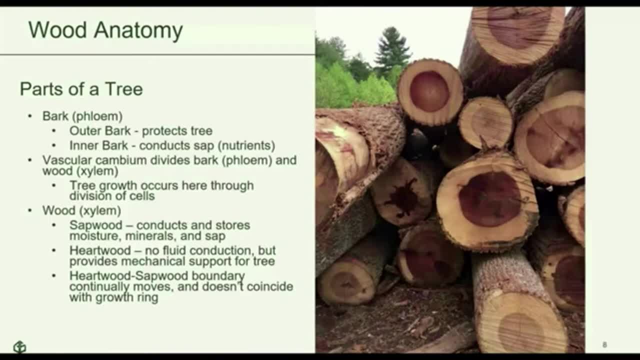 or oval. you know it's shaped in general kind of like the tree, but we've got some uh like like this one right here where the- uh, the heartwood, sapwood boundary has expressed some very interesting shapes. so it's again not something that that is constant and it's not something that coincides. 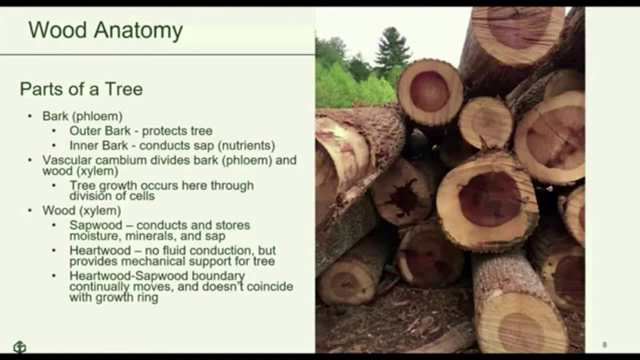 with a particular number of growth rings or anything like that. it's just something unique to the tree. the heartwood does contain extractives. these are the chemicals that give it the darker color that we can see present in this photo, and in certain species these extractives have. 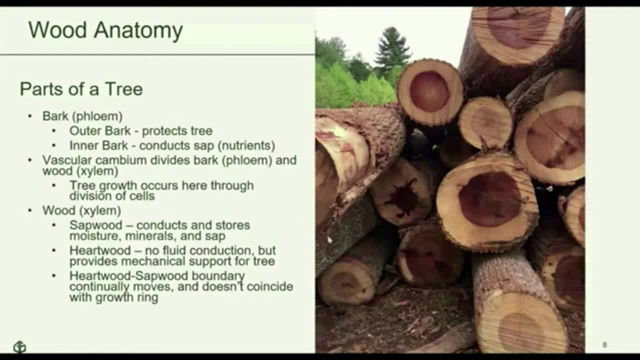 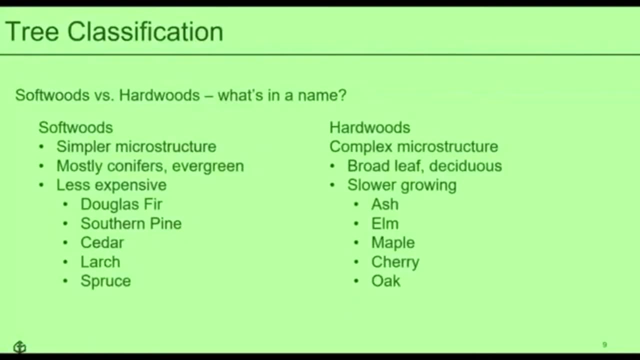 a great commercial value and are used for for all sorts of chemical processes. when we look further into the types of trees, we have two main classifications: we have softwoods and we have hardwoods and, despite what the name would imply, softwoods are not always soft and 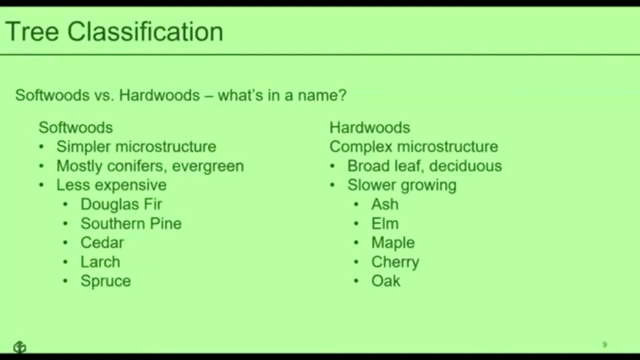 hardwoods are not always hard. softwoods are typically coniferous trees or evergreen trees. these are trees that don't lose their leaves in the winter. they'll have a very simple micro structure compared to to hardwoods and they do tend to be less expensive. these are are a lot of. 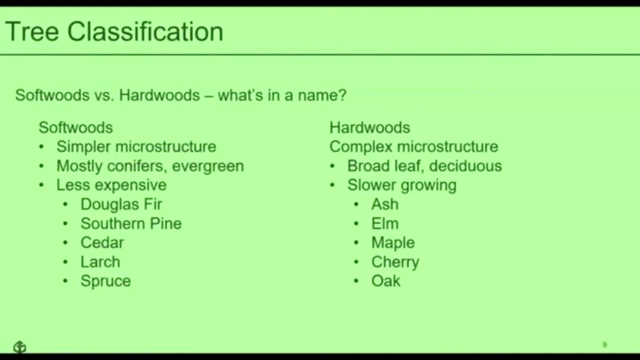 commercial species that we see for structural purposes. so things like douglas, fir, southern pine, larch and spruce trees. hardwoods are broadleaf trees or deciduous trees. these are trees that do lose their leaves in the winter and these trees typically will grow much more slowly than 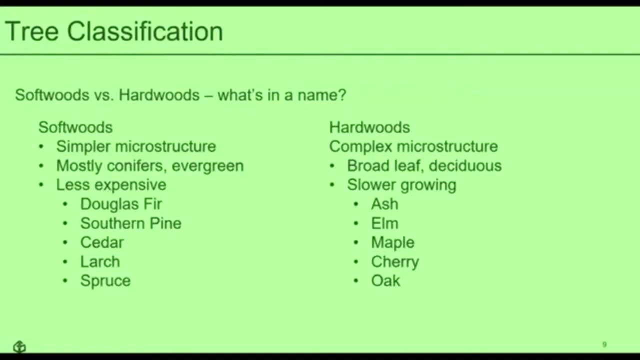 than softwood trees. some common hardwoods that we see in north america are species like ash, elm, maple, cherry or oak. these woods are typically prized for their appearance, so while they can be used for structural purposes, a lot of times we'll see them used in instances where their appearance can be uh brought forth. so you'll see them used a lot for. 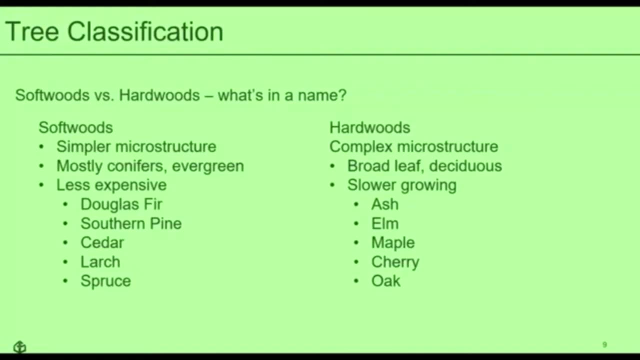 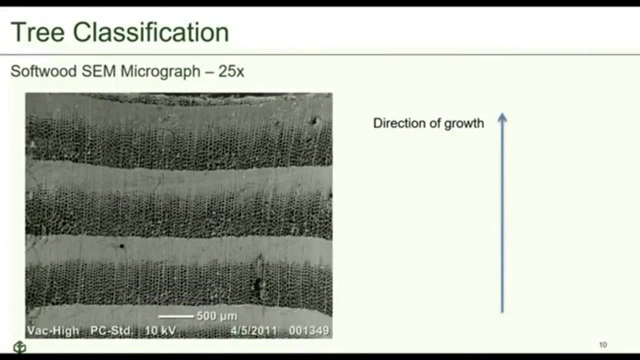 for things like furniture or for finishes going to our softwood scanning, electrical and other takeaways. so these are two species of softwoods we see here in north america and once we get into the south american woods we see that in these trees we're in these. 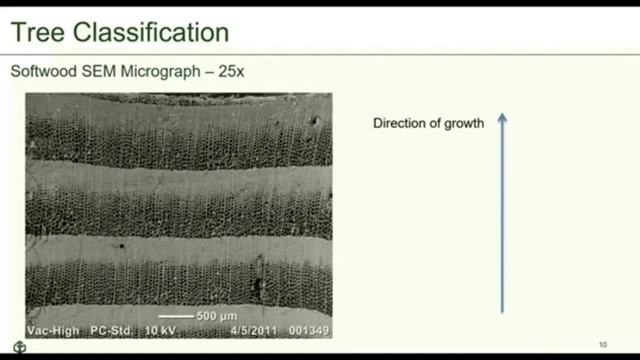 areas. we can see that this tree it's actually quite a lot longer. it's always a lot shorter. we can also see on a mycographic electron microscope micrograph. here we can see the direction of growth indicated here with with this blue arrow, composed mostly of the same types of cells. 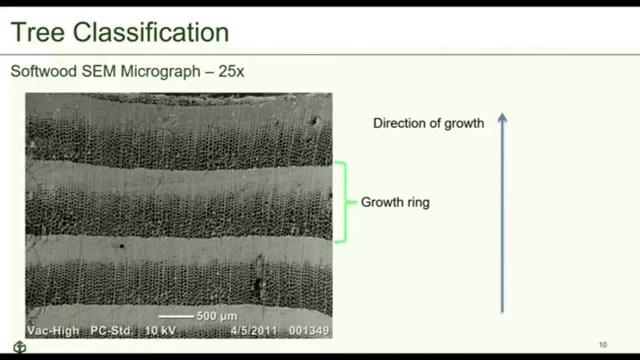 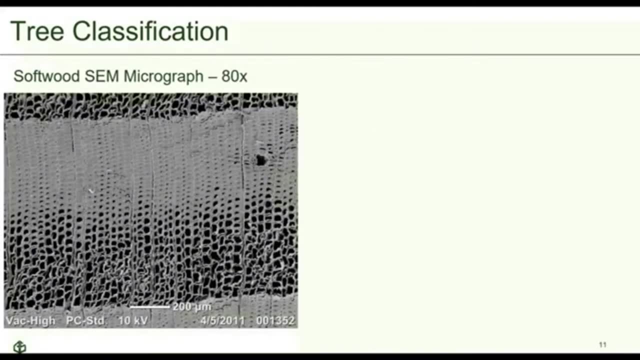 These are tracheid cells. We do see a little bit of variation, but for the most part it's a very uniform cellular structure. Zooming in a little bit more and looking at one individual growth ring, we see that we have two different parts of the growth ring. 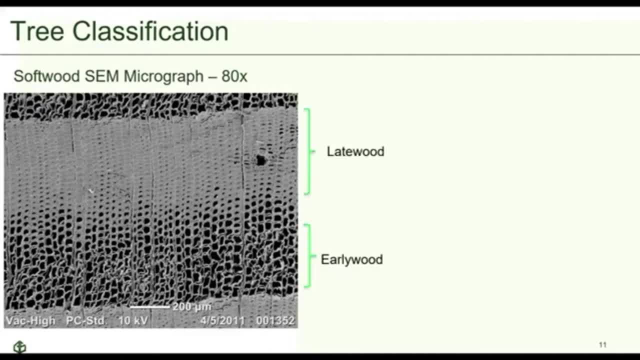 We have the early wood and the late wood And, as the names would suggest, early wood is grown early in the growing season, while the late wood is grown later in the season. We see the early wood cells have thin cell walls and in conifers this early wood production. 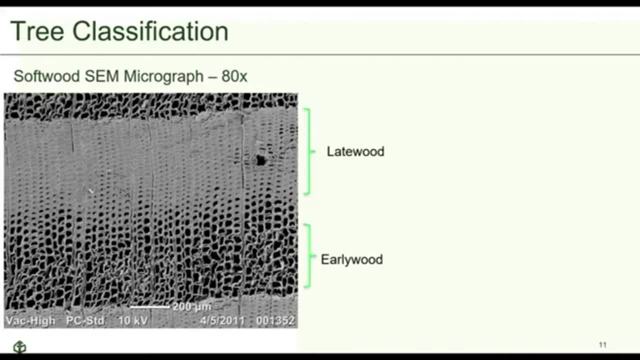 coincides with the tree's period of height growth. The late wood production is facilitated by the fact that the foliage, or the now mature foliage, in the crown of the tree, at the top it's producing a surplus of sugars that we can distribute to regions of active growth. 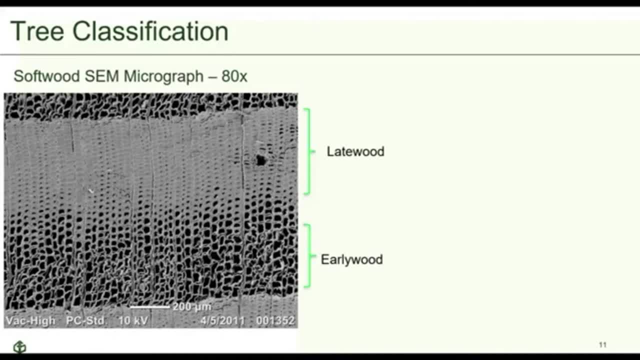 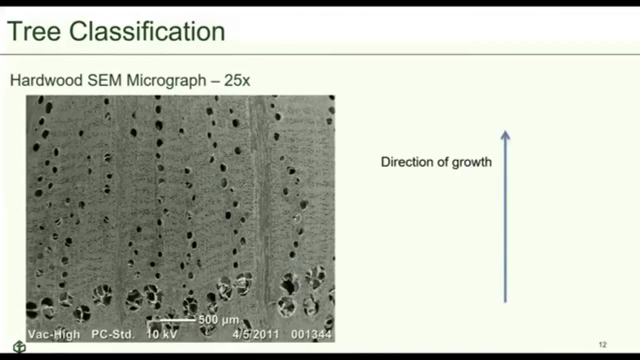 So we can develop these much thicker cell walls in the late wood. And because the late wood is so much denser, it has a much stronger impact on the mechanical properties of the wood. Thank you for joining us. Have a great day. Looking at now at a hardwood. 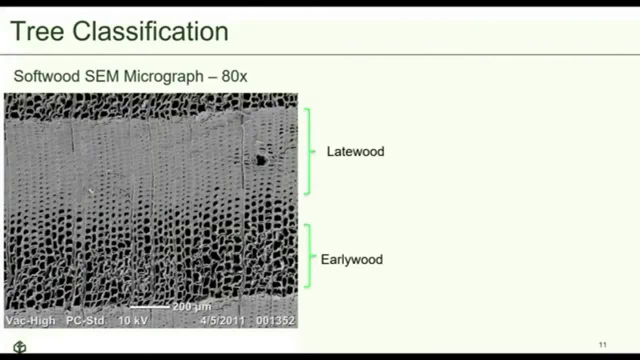 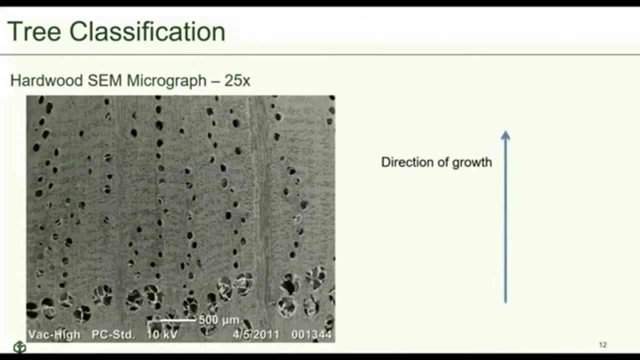 our previous slide here, this one was: this: softwood is a piece of pine. Now if we switch over to our hardwood scanning electron microscope micrograph, this is a piece of white oak And we can see a lot more variation in the types of cells in this cross section. 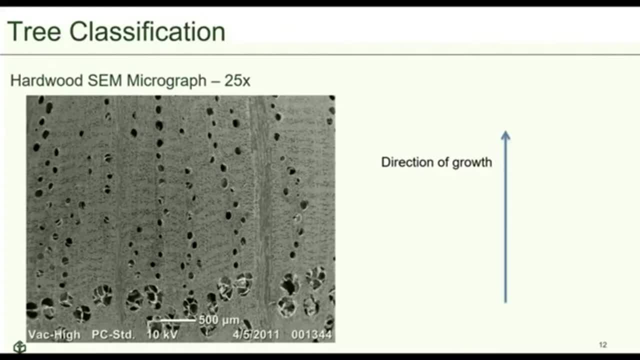 than we saw in the previous slides for the softwood. Again we see our early wood cells towards the bottom of the slide. here These are conduits for moving water and minerals from the root system to crown. So we see in the hardwoods these early wood vessels. 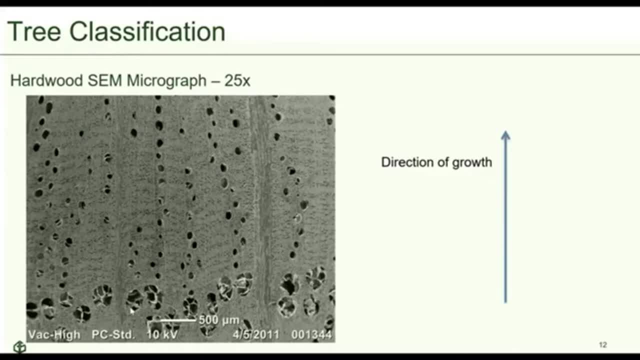 these large holes that are used to move minerals and nutrients during the early part of the growing season, And these early wood vessels in white oak and other species that are known as ring porous species can actually be identified with the naked eye. So one growth ring here. 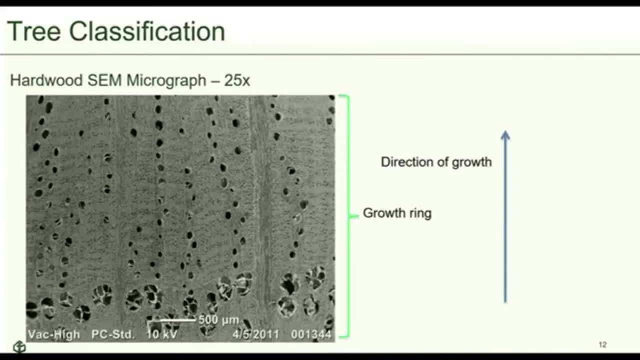 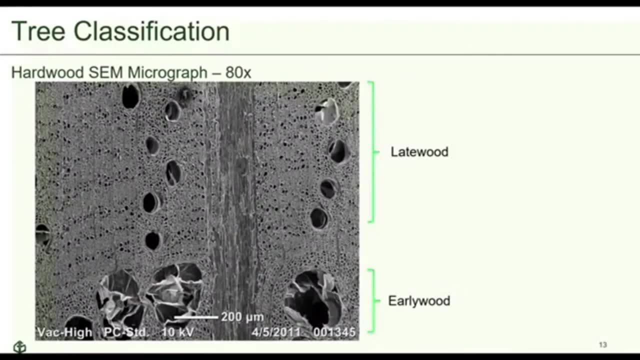 is represented in this section. So in this slide we see the variation of the different types of cells much more clearly. The early wood vessels again are much more pronounced. They're quite noticeable towards the bottom of this illustration, And the late wood vessels become smaller. 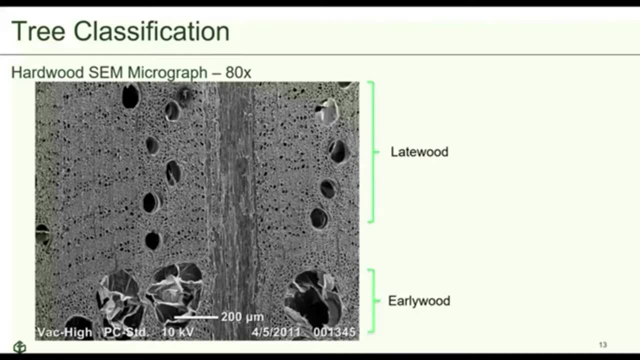 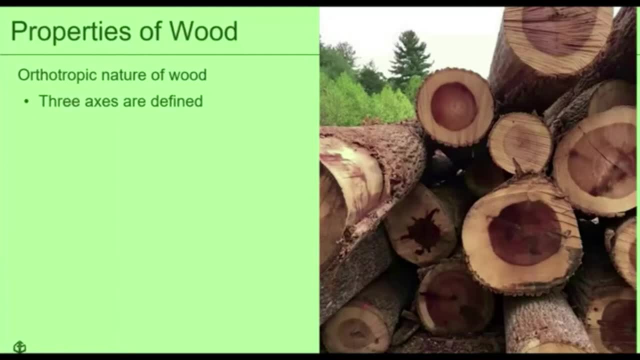 as water becomes more scarce later in the growing season. When we look at the different acts, we have three different axes we deal with. Because wood is an orthotropic material. We've got different axes and it will behave differently depending on the direction you're looking at. 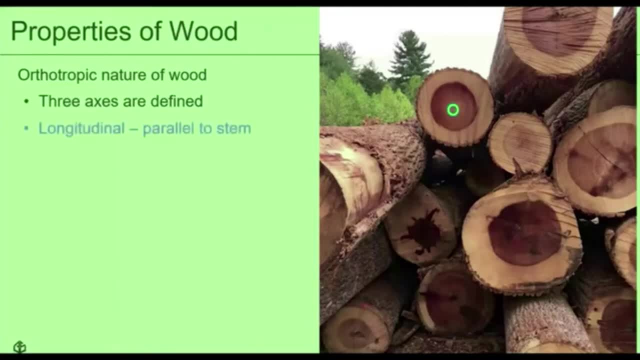 So we have the longitudinal axis, which you can see illustrated here with this small green circle. The longitudinal axis is parallel to the stem or the direction of upward growth. So in this picture for that log, the longitudinal axis would be coming out of your screen at you. 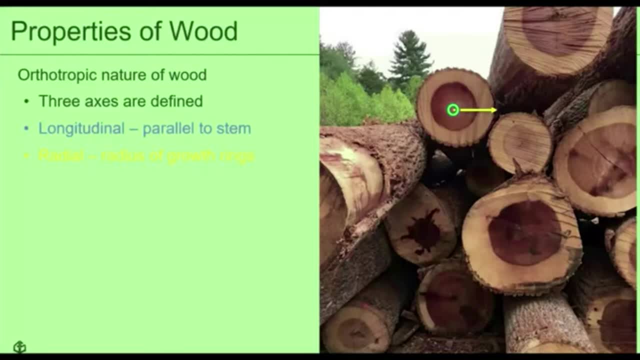 The second axis is the radial axis. So if we look at the cross section of the tree as if it were a circle and we drew a radius of that circle, the radial direction is what is represented by that. The third axis is the tangential axis. 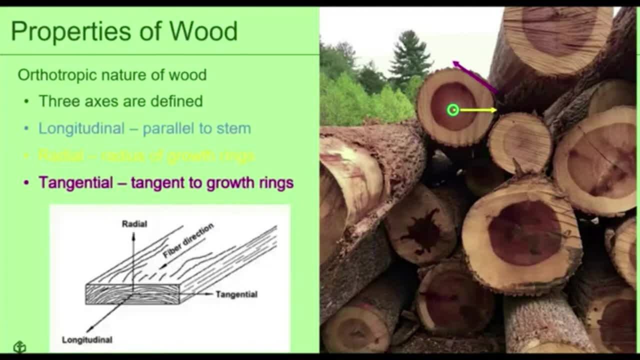 The radial axis is the longitudinal direction, So that would be a tangent to that circle created by those growth rings. And when we take a look at how this appears in a typical piece of lumber that we're looking at, we see the longitudinal direction is typically the length of the board. 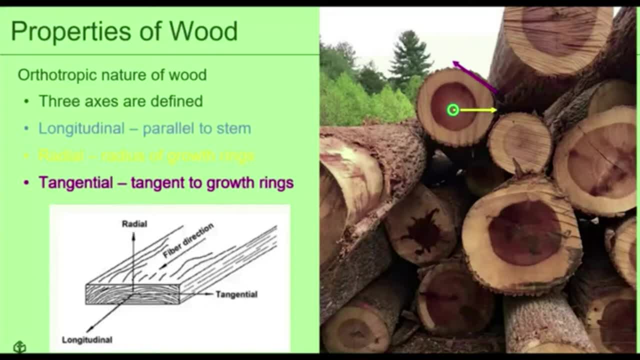 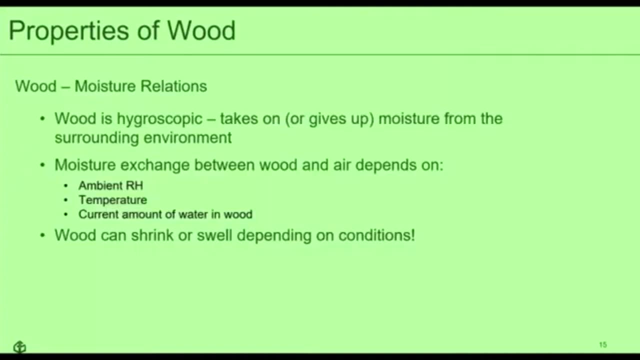 While the radial and the tangential directions are going to be expressed as the cross-section, the horizontal direction is the length of the board. there Wood is hygroscopic. That means it takes on or, in some cases, gives up moisture from the surrounding environment. 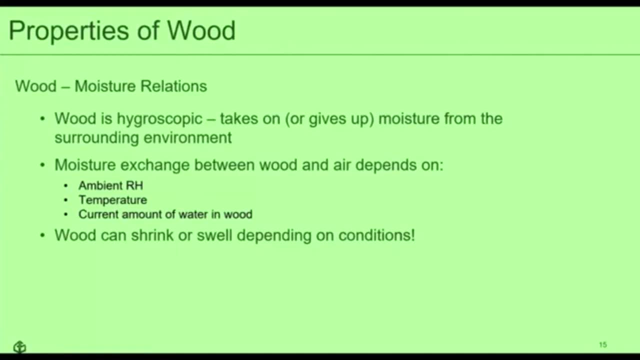 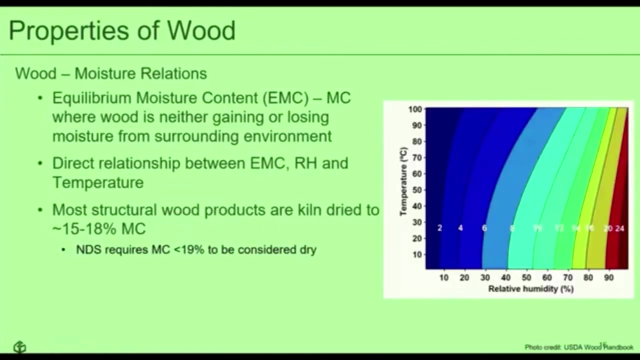 And that moisture exchange can depend on the ambient relative humidity present, It can depend on the temperature And it can also depend on the current amount of water present in the wood. So wood can shrink or swell depending on the conditions of the environment. The equilibrium moisture content is the moisture content. 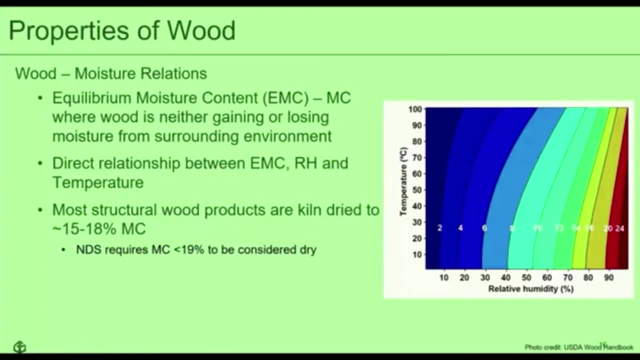 where wood is neither gaining nor losing moisture from the surrounding environment And, as you might guess based on what we just talked about on the last slide, there's a direct relationship between the equilibrium moisture content, or EMC, relative humidity and the temperature. 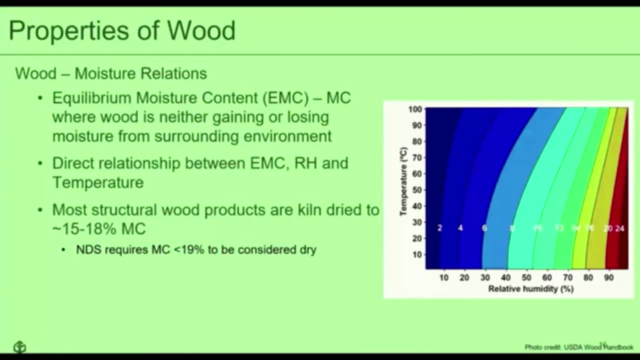 And we can see in this illustration here on the right side of our screen a graph from the USDA Wood Handbook that shows us what the equilibrium moisture content for a piece of wood would be for a given temperature and relative humidity. So if you're in a very high humidity environment, 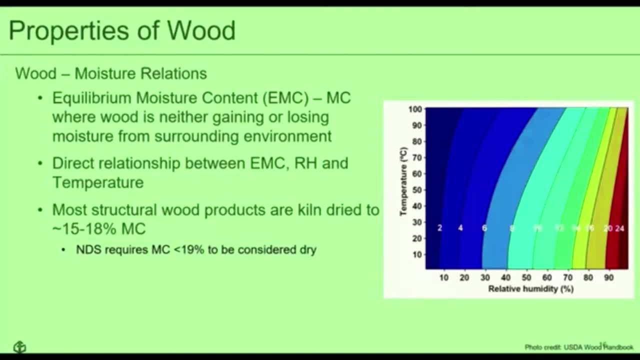 the equilibrium moisture content can be upwards of 14 to 16%. If you're in a low humidity environment, you see that the moisture content can be on the order of 8 to 10%. So why is this important? Because most structural wood products are kiln dried. 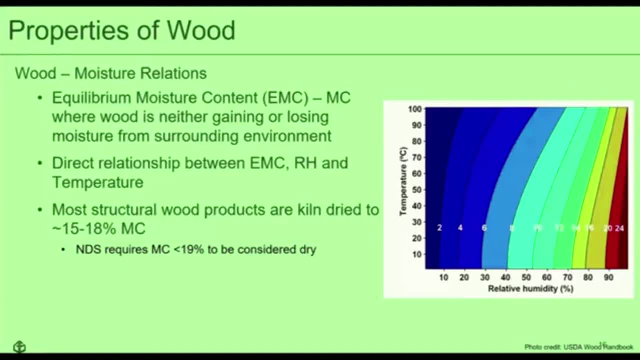 to about 15 to 18% moisture content. So when you lose that anywhere from you know 1 to 10% moisture content as your lumber equilibrate, you will have some dimensional change that can occur. The NDS, or the National Design Specification. 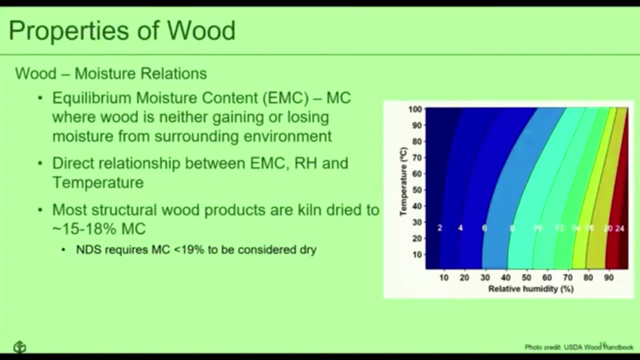 requires the moisture content for lumber to be less than 19% to be considered dry. So that's why we see that 15 to 18% target for our kiln drying, because it'll meet that minimum of sub 19%. How do we calculate the moisture content of wood? 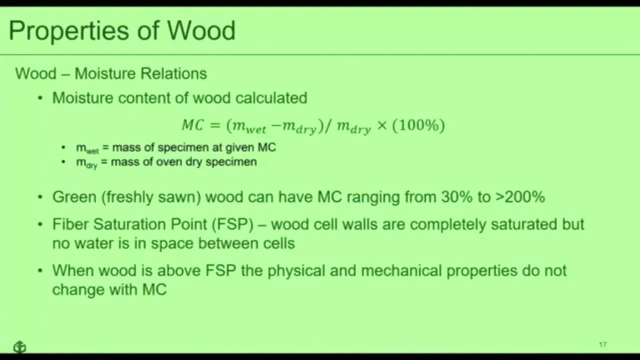 It's based on the mass at a given moisture, where we're trying to calculate what the moisture content is as well as the mass after the specimen's been oven dried. So freshly sawn lumber can have a moisture content ranging from anywhere from 30% to. 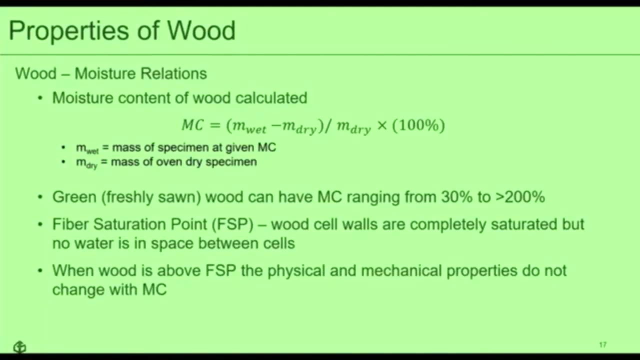 upwards of 200%, But again, when we're using the lumber we dry it to under 19%. There is a point known as the fiber saturation point, where the wood cell walls are completely saturated with water, but no water is in the space between the cells. 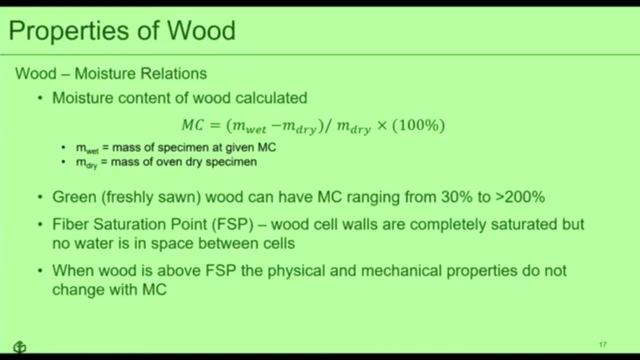 So when the wood is above the fiber saturation point, the physical and the mechanical properties don't change with the moisture content. So that basically means that those wood cell walls have absorbed all the water they can. If any more water is going into the wood, it's being stored in between the cells in the space between the 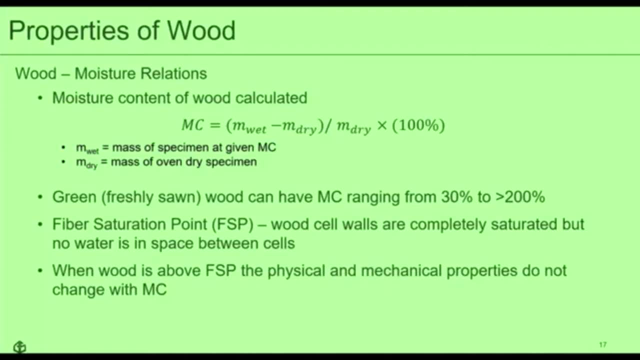 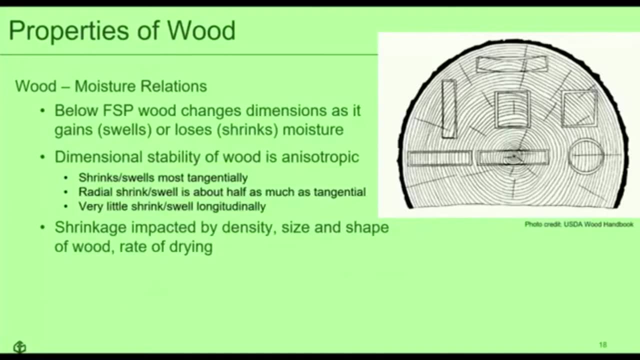 cells. So the wood won't swell any further beyond its fiber saturation point. That's as big as it can physically get. When we are below that fiber saturation point, which is where we typically will hang out as structural engineers, the wood will have been dried below the fiber saturation point. 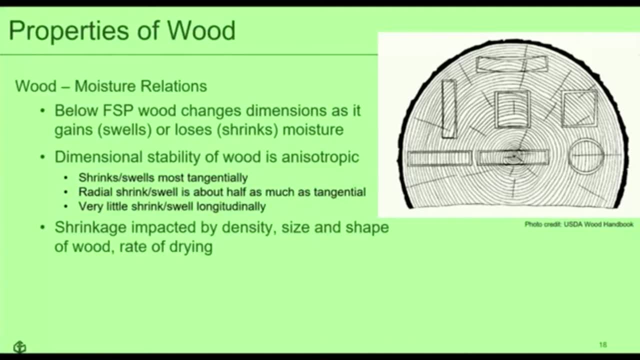 The one thing that matters here, that I'm going to show you, is that the fiber saturation tweaks a lot of different things. So one of the things that I'm showing you is a 3D print project, which is 3D printing. This is much more complicated and more complicated than what you may think, and this is not going. 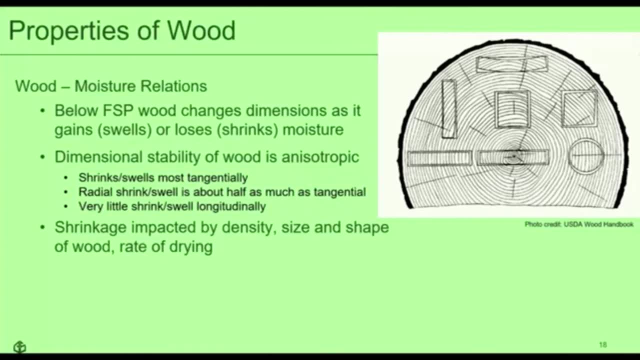 to be a simple fine print or full growth kit. This is Kennethabe scowling's project Right He's doing on him. content changing will occur in the tangential direction. The radial direction will have about half as much shrinking or swelling as the tangential direction, and then we see very 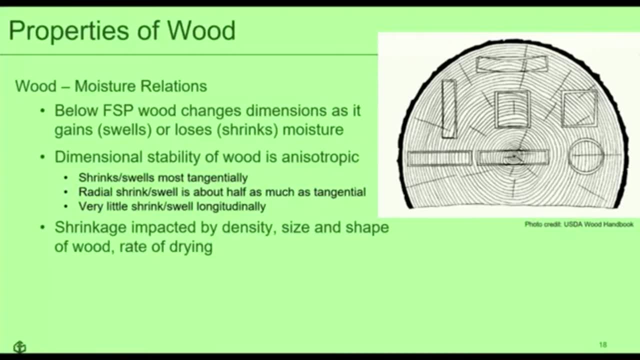 very little shrinking or swelling occurring longitudinally. The shrinkage is going to be impacted by a lot of different factors. It'll be impacted by the density, by the size and the shape of the wood, the rate of drying where in the tree it was cut from, and we can see that the 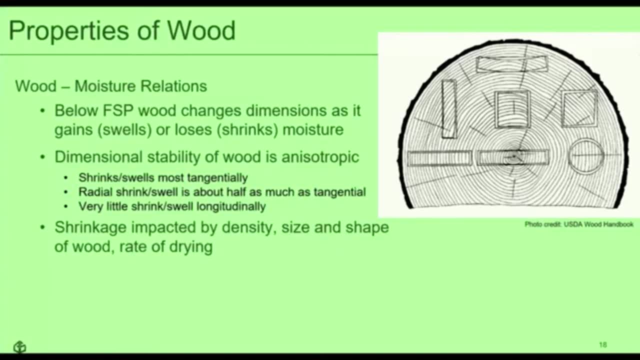 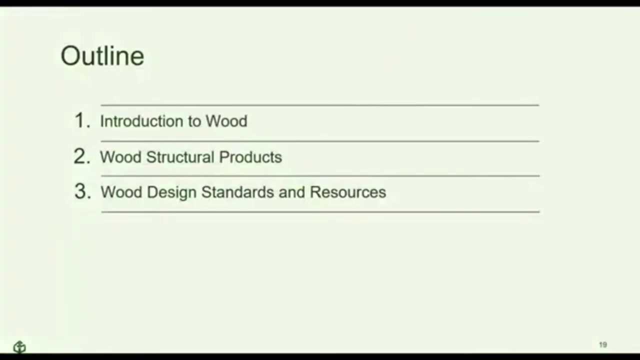 illustration here again from the USDA wood handbook can give us an indication of the influence on where in the tree a piece of lumber came from and how that can influence the shape it would shrink and swell in with regards to changing moisture. All right, Next we're going to move in and talk about some wood structural products. 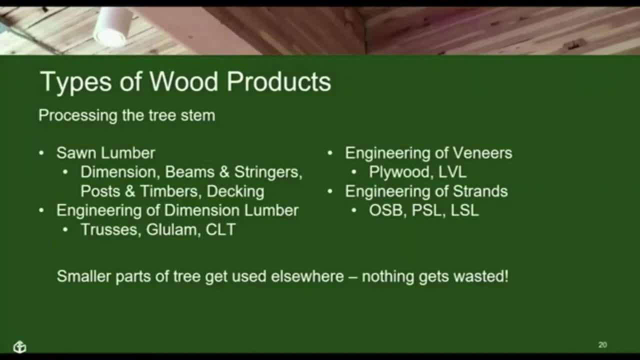 So when we process the tree stem, we have a lot of different things that get made. We start with sawn lumber, So these are our familiar elements, our dimension lumber, such as two-by-fours or four-by-sixes or things like that. 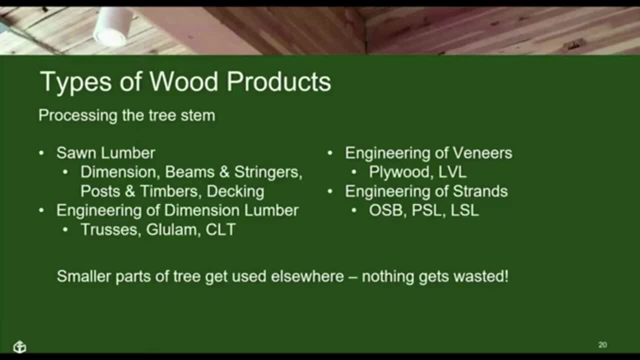 We also have beams and stringers, posts and timbers and decking, and we'll talk about the difference in classifications between those different elements. When we start engineering dimension lumber, when we start making bigger things out of it, we produce things like trusses. 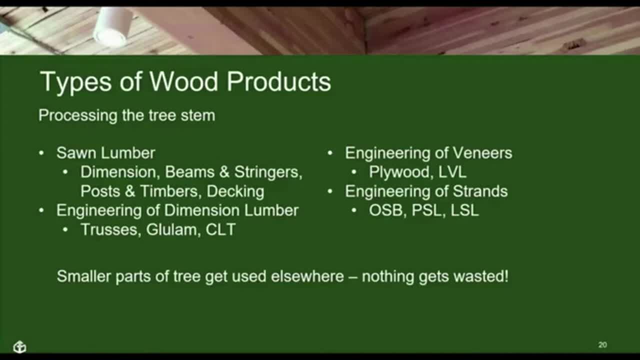 glue-laminated timber or glulam, or cross-laminated timber or CLT. Sometimes we'll make the wood into pieces that are smaller than our dimension, or sawn lumber, So we'll use products such as veneers. A veneer is produced by taking a 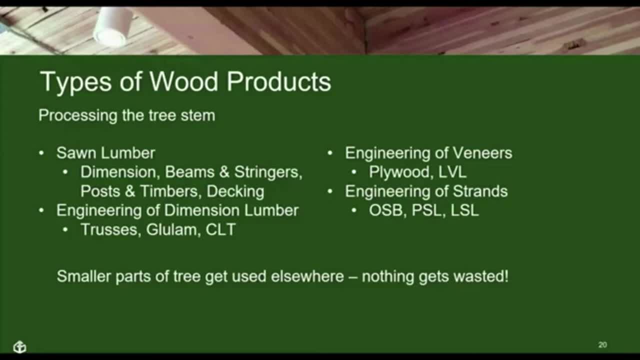 log and putting it on its side and you put a blade against it and you kind of unroll it similar to a roll of paper towels. So we use these very thin veneers of wood and make products like plywood or LVL, which is a laminated veneer lumber. 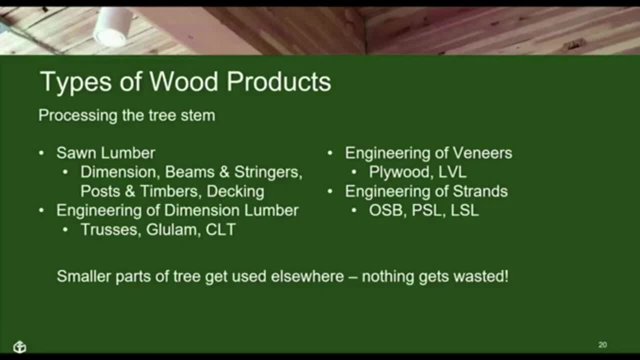 Engineering smaller elements like strands, where the veneers or smaller pieces of wood are chopped up. We get products like OSB oriented strand board, PSL parallel strand lumber or LSL laminated strand lumber, So the smallest parts of the tree will get used elsewhere. 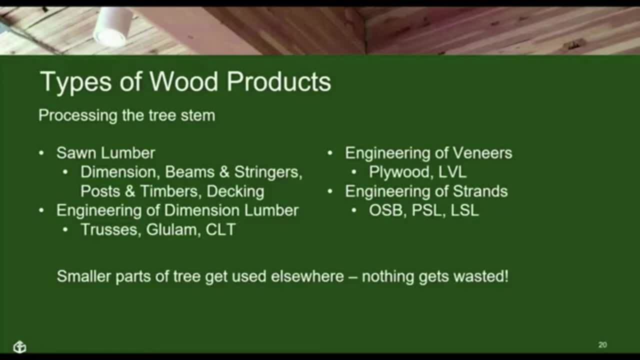 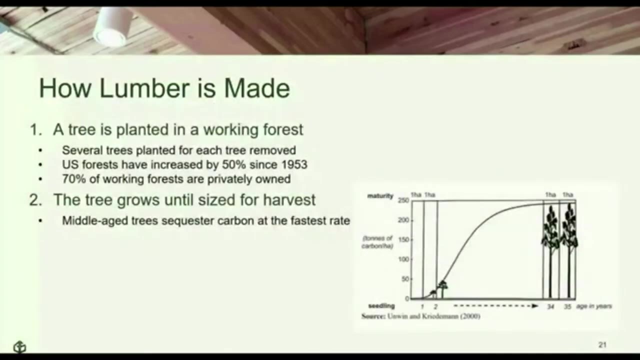 Nothing is getting wasted. We have parts that go to paper and packaging industry production and some that's used for energy production, So absolutely nothing from a tree that gets cut down is going to waste. So how do we get these trees and how do we turn them into lumber? 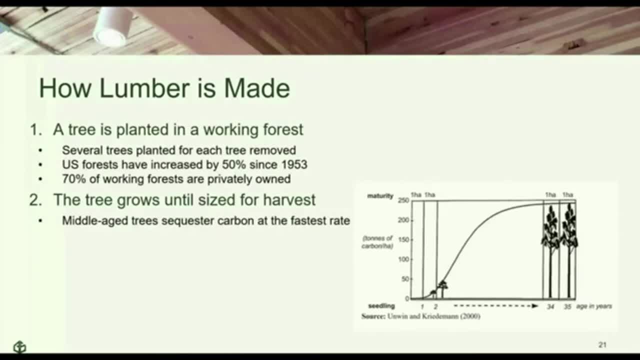 So first the tree is planted in a working forest. As I mentioned, we plant several trees every time we remove a tree from the forest. The US forests have increased in size by 50 percent since 1953.. The tree will grow until it's sized for harvest. 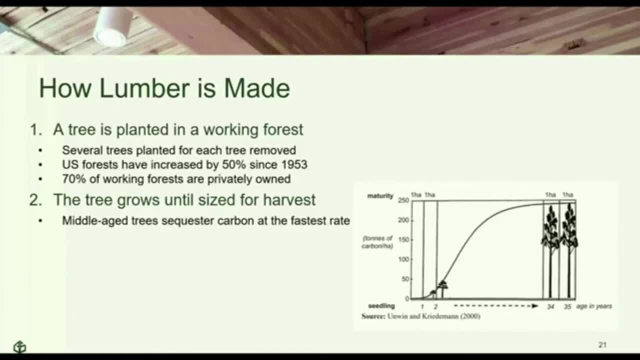 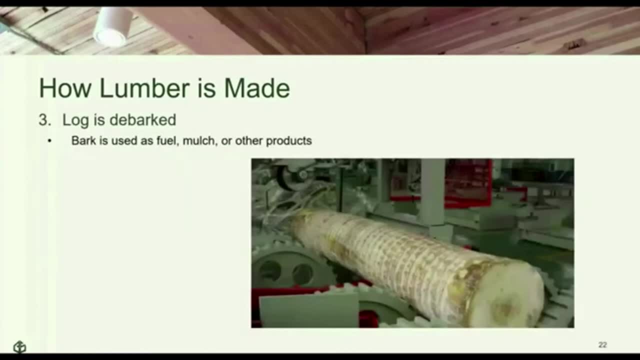 and actually middle-aged trees. we see sequester carbon at the fastest rate. Once the tree is ready to be harvested, it's cut down and it's taken to the lumber mill where it's debarked. The bark will be used for things like fuel or mulch or other products. 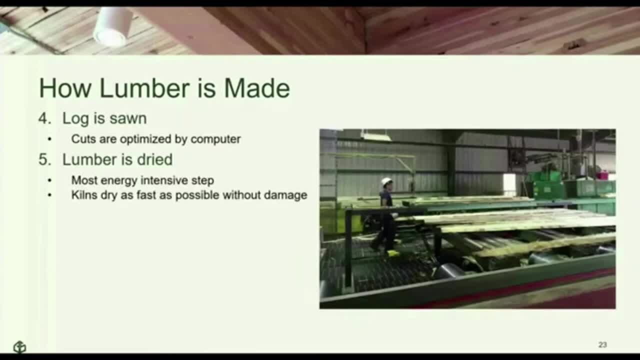 And then we saw the log. The cuts in a given cross section are optimized by a computer. So it's all done with computer guides and laser accuracy, and it's a very impressive setup if you've never been to a lumber mill. The next step is drying the lumber. So we talked. 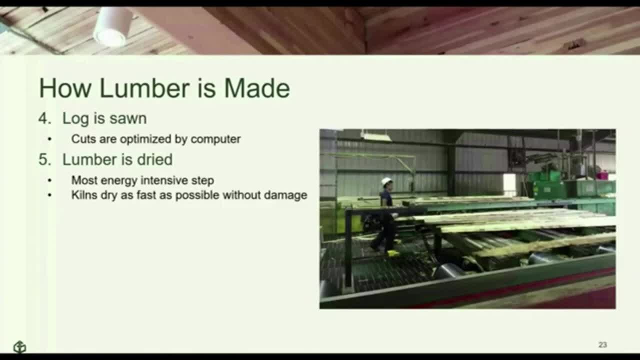 about how. when lumber is cut, the moisture content can be very high, but we need to get it below 19% for it to be considered dry. So this is actually the most energy intensive step in the production of lumber, and we use kilns to dry the lumber as fast as possible without damaging the lumber. 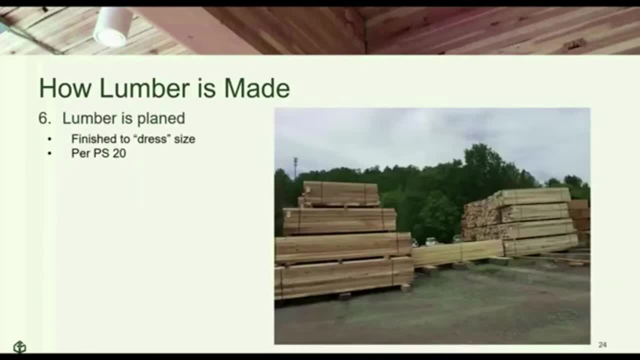 So once the lumber is dried it's planed and finished to its dress size, and the dress size is specified in standard PS20.. So a two by four nominal is actually one and a half inches by three and a half inches. 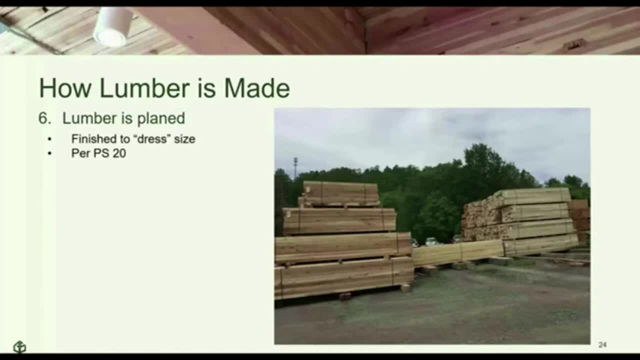 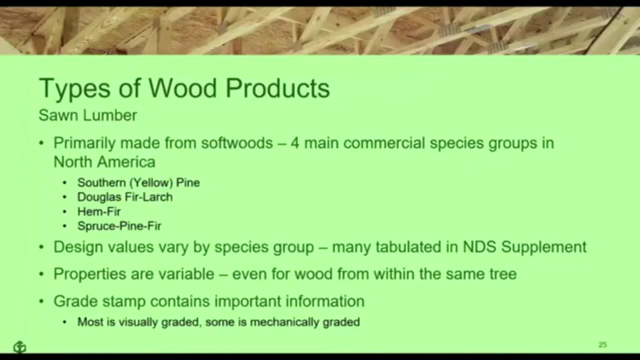 Those types of dimensions and sizes. that's all specified in PS20.. So when we talk about our sawn lumber, we have four main commercial species groups in North America. We have Southern Yellow Pine or Southern Pine- the term can be used interchangeably. We have Douglas Fir, Larch. 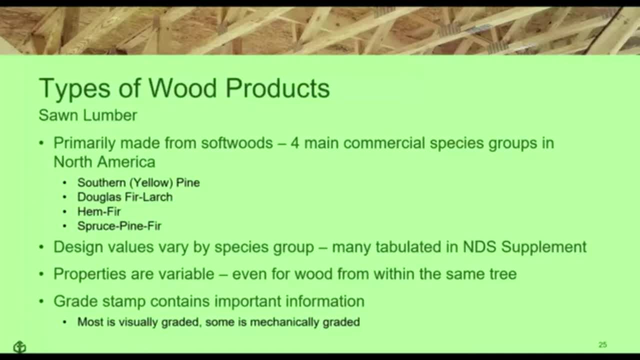 Hem Fir and Spruce Pine Fir, And you see some of these that contain more than one species of tree and you might wonder why is that? And that's because out in the forests, these are species of trees that are commonly growing in the same stands. They grow together. 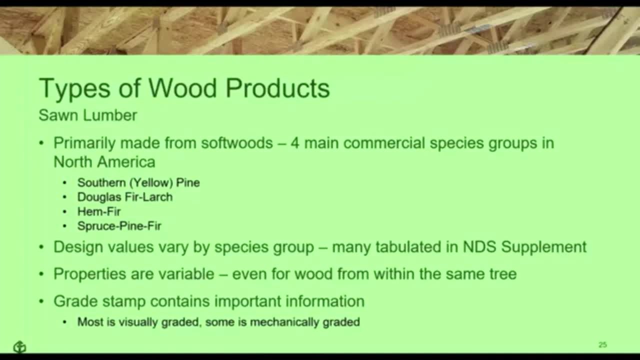 So rather than just going through and picking out individual Douglas Firs and leaving Larch, or vice versa, that they will harvest all of them and it becomes a commercial species group. So the design values do vary by the species group And in the NDS supplement we do have 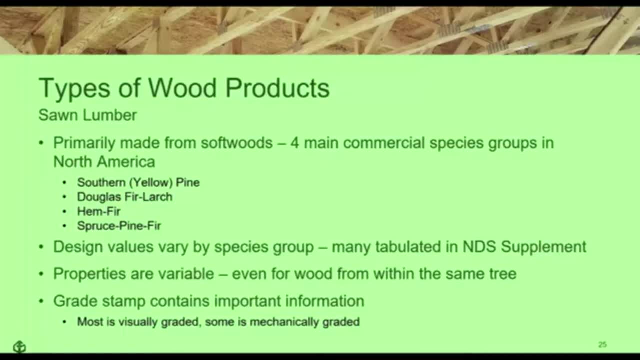 many of them tabulated. So most of them are North American species, but there are also non-North American species listed in the supplement, And the properties for wood can be variable. You see your combination of two, acid and four matter, tartdom, So that one is the parent species and the other is that one that you didn't have in the plan And you now have the type on the dead ass of the tree. Now, one of them will simply be a tree. This means that you don't need to trap it, But you can tag along another plants or karış in a row or take it some where else. Alors, most spiderbrurs are able to be in the same way knows how they can hide the plant in the Serving tree. 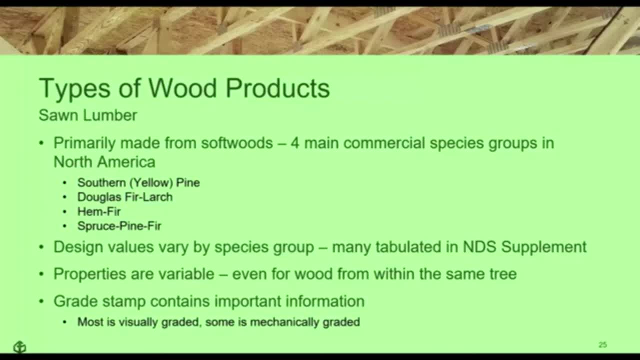 and the properties for wood can be variable, even for wood within the same tree. so that's why we grade the lumber, and we'll talk about that in a moment here. but all lumber will have a grade stamp and that grade stamp is going to contain really important information like the, the grade, 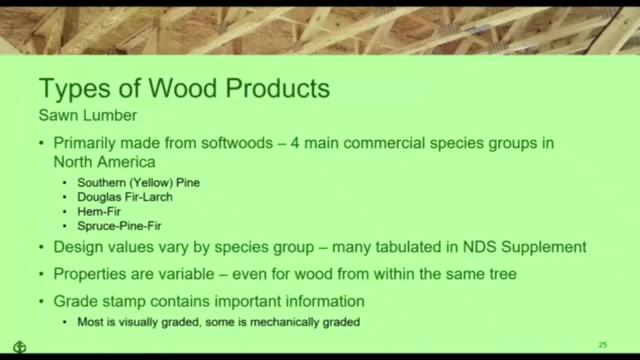 where the mill identification of you know where that lumber was processed, the grading rules that were used to grade that lumber is. that's all going to be contained in the grade stamp. most lumber is visually graded. that means somebody looks at the actual board and and decides what. 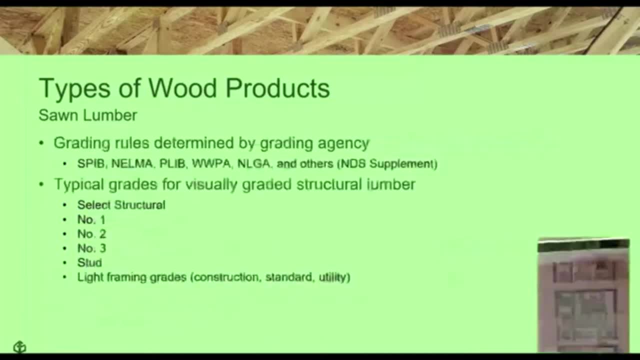 the grade is, but some is mechanically graded. the grading rules for lumber are determined by a grading agency and we have several listed in the the NDS supplementation. some of the the bigger ones are SPIB, the southern pine inspection bureau or the western wood products association. there are various agencies out there and you can take a look at their, their. 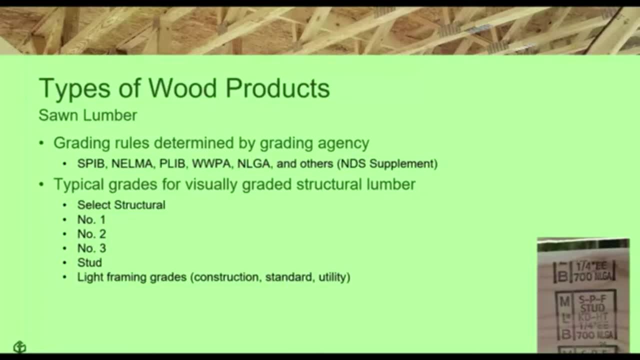 information in the NDS supplement if you have questions on anything related to that. the typical grades we see for visually graded structural lumber: our select structural is: is the cream of the prime grade Kobe beef, the the best grade material, and then number one, two and three as 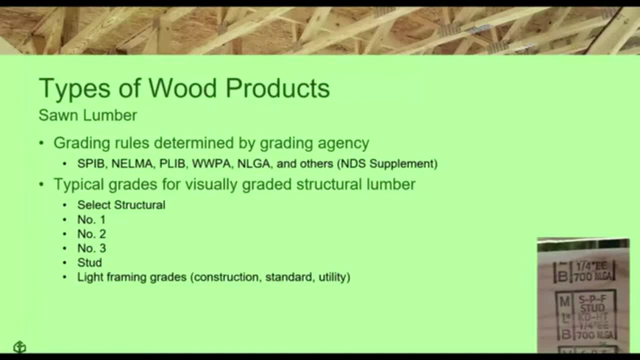 well as stud. we also have light framing grades such as construction standard and utility grades. when, when an examiner looks at a piece of lumber for visual grading, they'll examine surface features, uh checks and things like warp and crook and other strength reducing characteristics and that could. 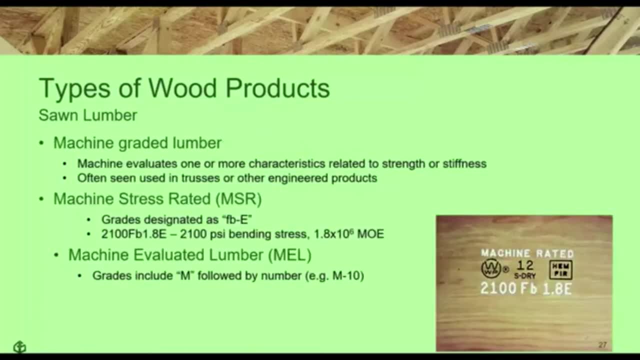 impact the the product. looking at machine graded lumber, a machine will evaluate one or more characteristics related to strength or stiffness. this is going to be done in the linear elastic region, so these are all non-triangular and non-triangular. so these are all non-triangular. 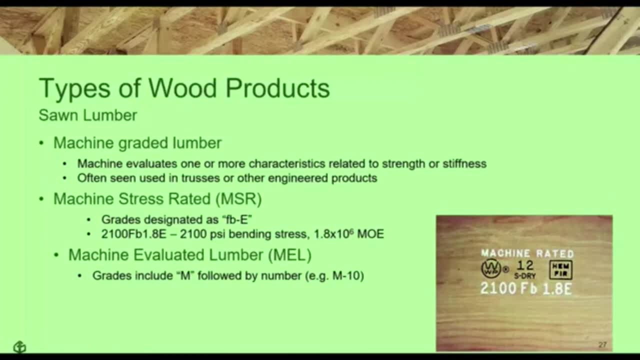 destructive evaluations, so there isn't any any damage, that is, that is done to the the lumber in the machine evaluation process. we'd see these products used commonly in trusses or other engineered products. the two primary types of machine graded lumber that we we see specified in the NDS are machine stress rated lumber or MSR, and that has 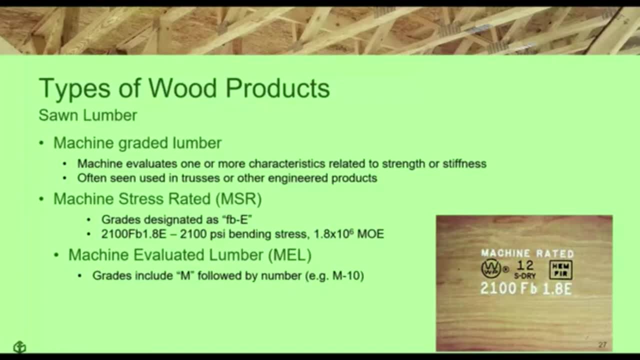 its designated as an FB-E and that's your bending stress and your modulus of elasticity. so in this illustration here we see an example of a machine rated grade stamp that shows a 2100 FB 1.8 E stamp. that means the bending stress in it on for this lumber is 2100 psi and the modulus of elasticity 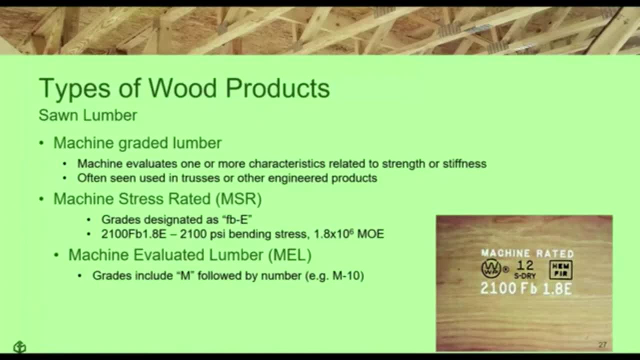 is 1.8 times 10 to the sixth psi or 1.8 million. machine evaluated lumber has a slightly different grading. uh nomenclature. you'll see this lumber graded with the letter M followed by a number, so a grade might be like an M10 or an M8 or something like that. when we talk about the different types, 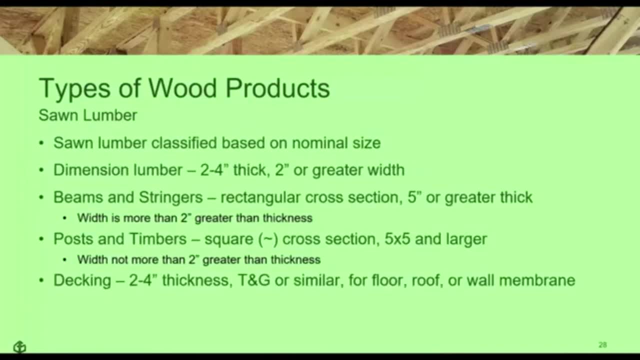 of sawn lumber. uh, it's classified based on the nominal size. so dimension lumber is a common, common type that we would design with where the lumber is two to four inches in thickness, uh, and two inches or greater in width. so, as I mentioned, you know, two by four. 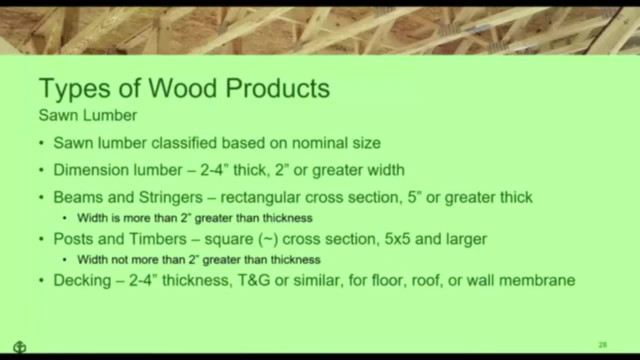 um four by sixes, lumber like that. uh, beams and stringers- these are slightly larger. these are sort of a rectangular cross section that are five inches or greater in thickness where the width is two inch more than two inches greater than thickness. so if you had a larger member, like a 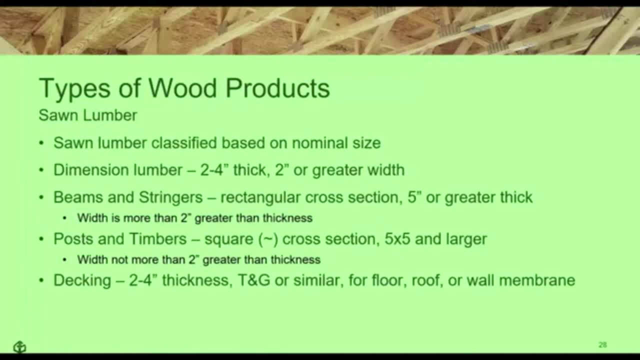 six by ten. so these again are more rectangular, uh, in in nature. posts and timbers again are are also larger. uh, cross sections, um, they are five by five and larger again, those are the nominal sizes. uh, for posts and timbers the width would be not more. 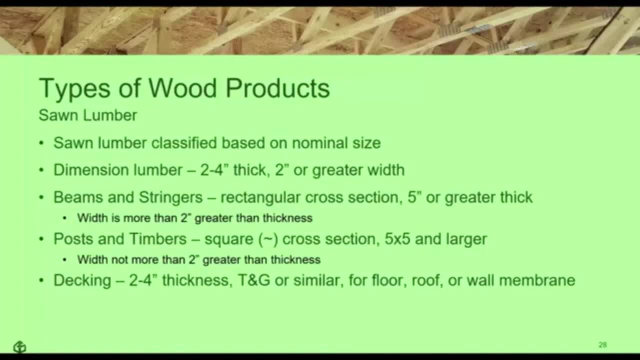 than two inches greater than the thickness, so something like a six by six or an eight by eight would be classified as posts and timbers. and finally we have decking. this is two to four inches in thickness, and sometimes we see tongue and groove or TNG decking, uh, or similar decking. 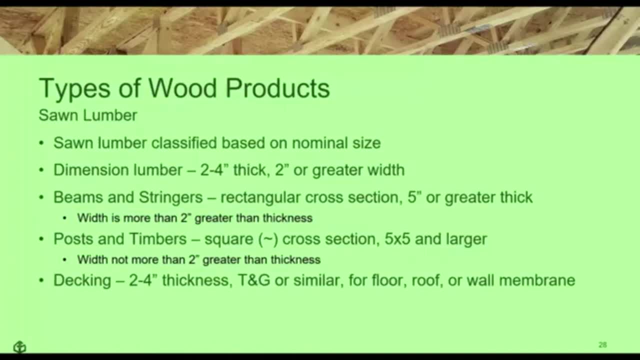 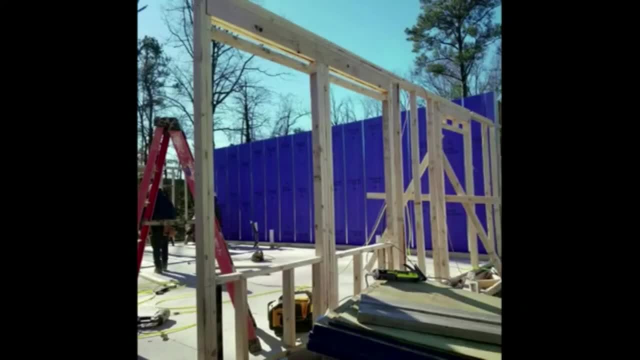 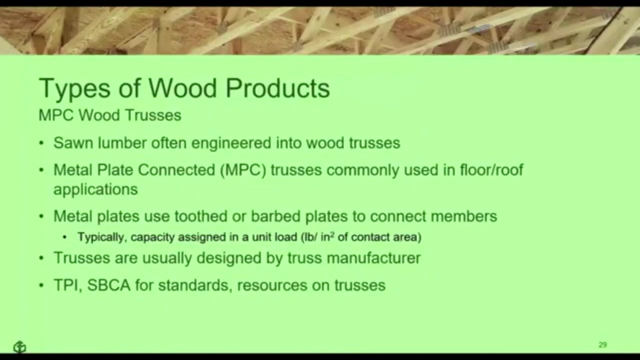 for floor, roof or wall membrane uses- and this is just a illustration of a wall in a townhouse. it's actually my townhouse that I live in, uh that that uses uh nominal two by four sawn dimension lumber in the wall framing. so I briefly alluded to uh mechanically evaluated lumber and machine. 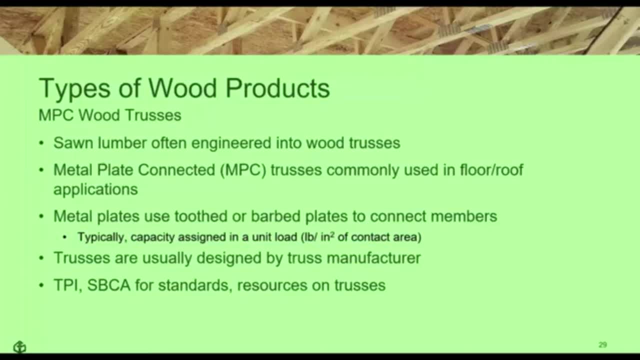 lumber sometimes being used in wood trusses. uh, the most common type of wood truss we see is are known as MPC wood trusses or metal plate connected. these are trusses that are commonly used in floor and roof applications and the metal plates used to connect the elements used toothed or barbed plates. 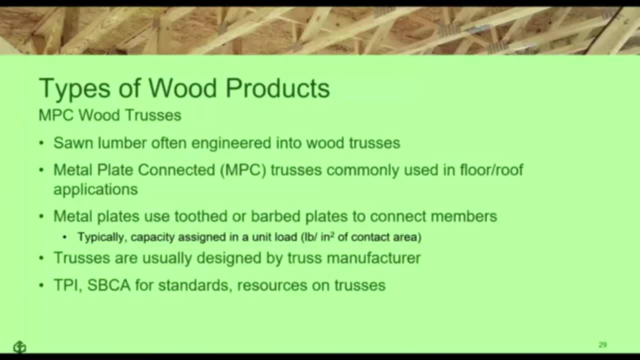 to connect the members uh the. the capacity on these types of fasteners, connectors, is assigned based on a unit load or, you know, the, commonly the pounds per square inch of contact area in a given connection. these are typically going to be designed by the truss manufacturer, so a vast majority of us will probably never design. 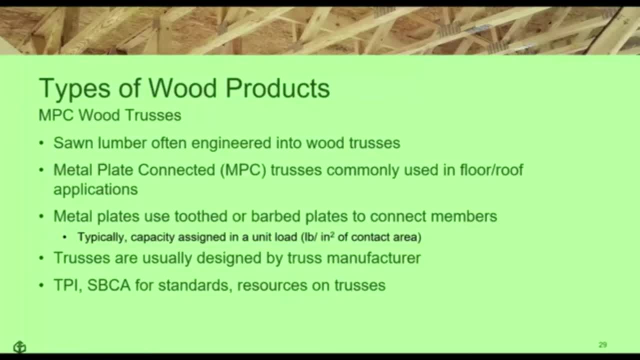 uh, an M metal plate connected truss. but if you are working for a truss manufacturer uh or doing some evaluations or something you, you may come across uh one of these and you might need to evaluate something. so we recommend taking a look at TPI the truss plate. 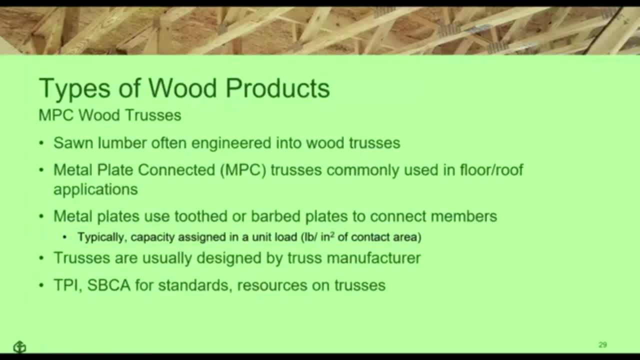 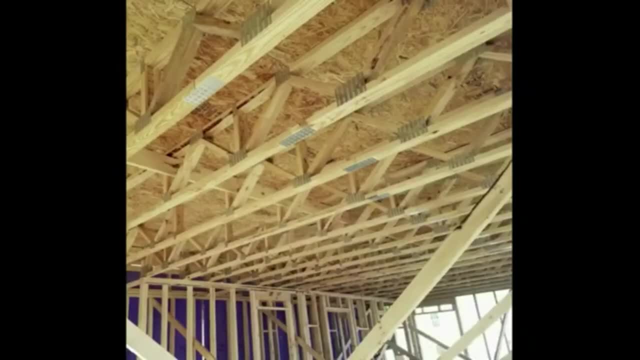 Institute or sbca, the structural building components Association, uh for for standards and different resources. on on trusses. and here's a another illustration of uh, my townhouse under construction. these are the parallel cord trusses that are used for the floor ceiling assembly between my first and second floor. the next uh structural product. 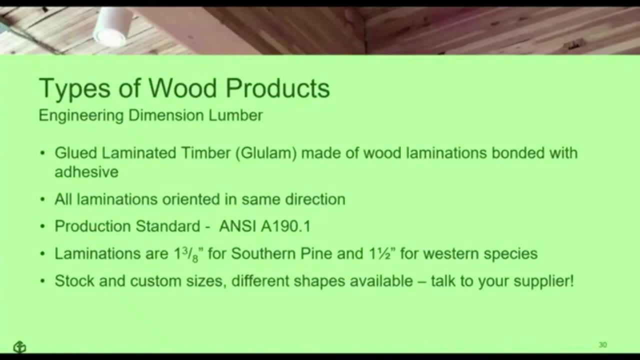 we're going to talk about it. that's made of Dimension, Lumber is glulam or glued laminated timber, and this is where we have wood laminations bonded with an adhesive, and for glulam products, all the laminations are going to be oriented in the same direction, so 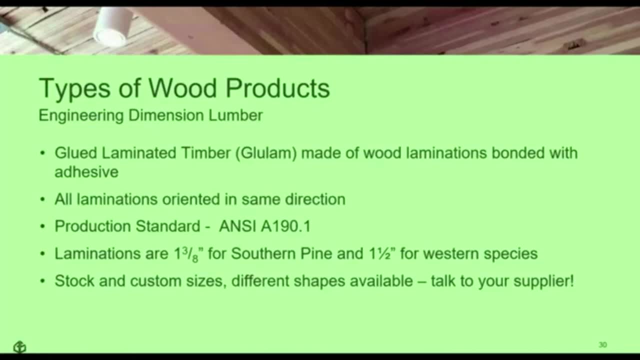 you'll typically see these elements used as beams or columns. you know something where they're carrying load just in one direction along the length of the member. the production standard for glulam is antsy a190.1, so that contains all the rules and regulations and such. 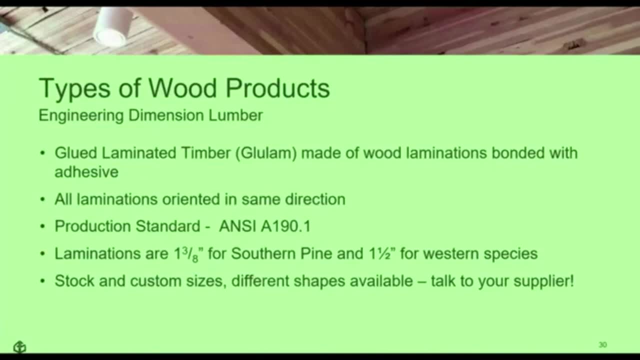 laminations that you'll see for glue laminated timber are different depending upon the species. so for Southern pine or Southern yellow pine the laminations will be one and three-eighths inch thick and for Western species, typically Douglas fir, you'll see the laminations are an inch and a half. 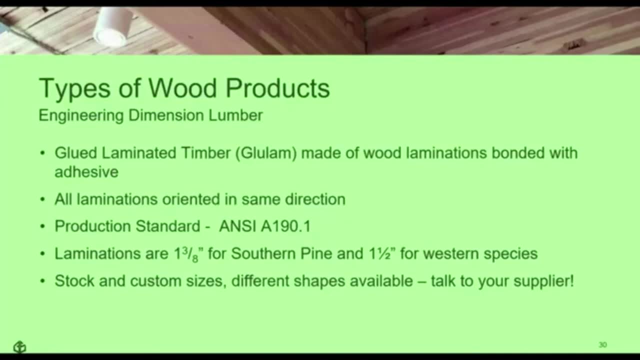 uh, and the reason is is, when the Southern pine material is is dried uh in the kiln, uh, sometimes it will uh secrete a little bit extra sap and that can interfere with the adhesive bond. so the suppliers, uh, the manufacturers, will plane off that. that, just that one-eighth of an. 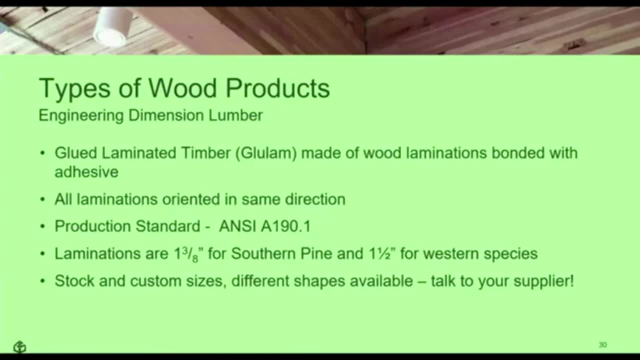 inch uh to take care of of that sap that might be on the surface. uh for for the Southern pine. so that's why we see the difference in the lamination thicknesses. um uh can be ordered in stock sizes. there's a variety of sizes that are standard, that many 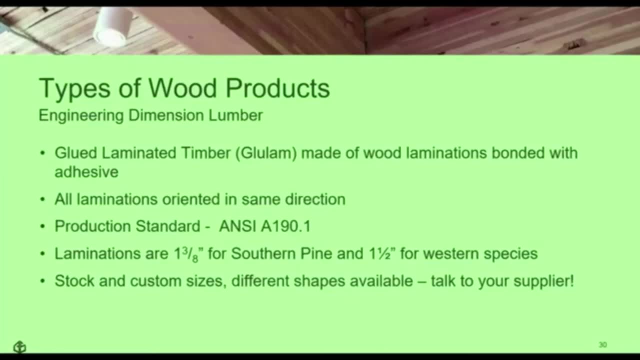 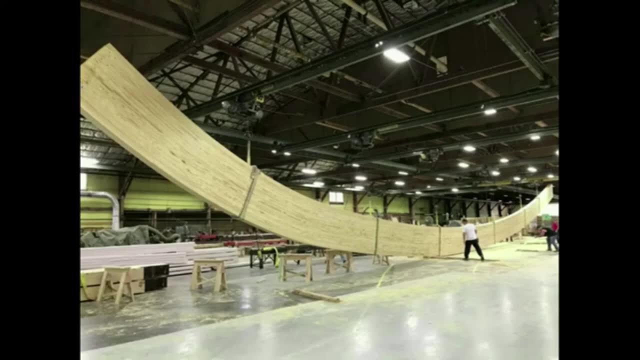 manufacturers will have readily available. you can also order custom sizes or even different shapes. um, here's a pretty impressive glulam Arch that our friends at unilam that produced at their factory up in New York. so again, um, you know, this is something that's. it's an impressive structure you'll want to work with. 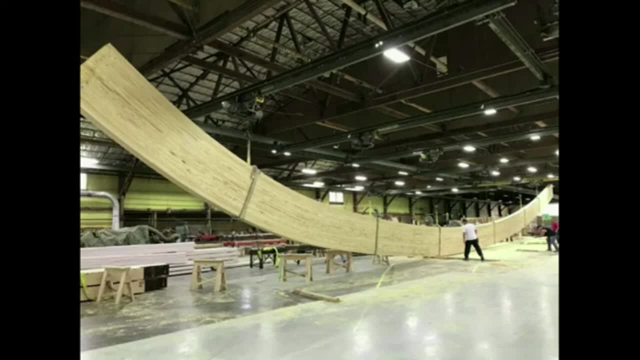 your supplier if you're going to be doing something unique like this, but if you are just trying to to get something that is, uh, a glulam beam and in a smaller cross section that you know the the lead time on those would typically be a lot less than on something custom. 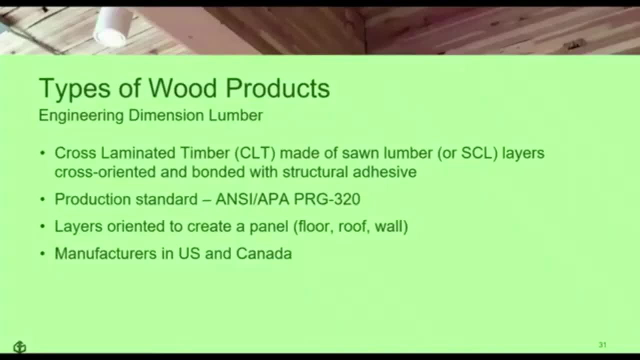 like this. so if we take this- a similar principle to glulam- but instead have the uh oriented into panels instead of all the members oriented in one direction, we get cross laminated timber. so CLT is made of sawn lumber or sometimes structural composite lumber layers that are 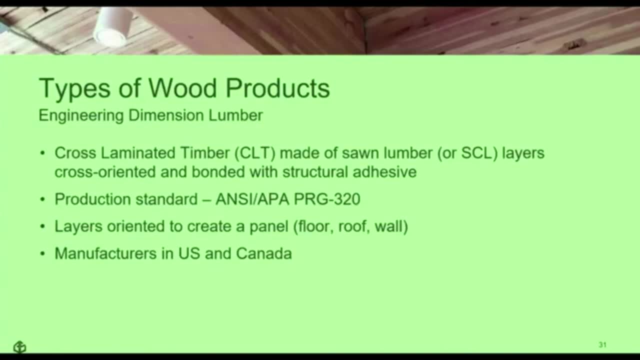 cross-oriented and bonded with a structural adhesive, and typically the way they're produced is each layer is 90 degrees or it's orthogonal to the adjacent layer. the production standard for cross laminated timber, or CLT, is APA PRG 320 and the layers uh oriented are or oriented. 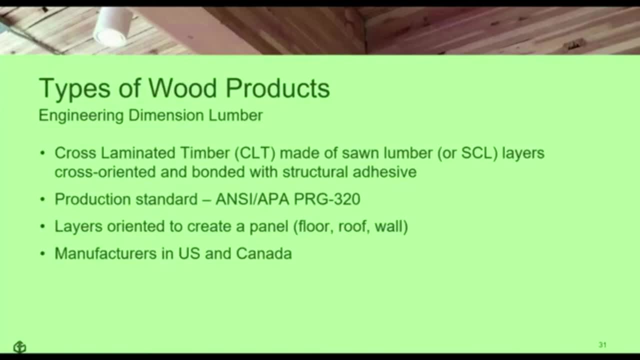 to create a panel that can be used for floors- uh, for roofs and for walls, so you can create an entire building out of this stuff. it's a really cool product. there are manufacturers in both the US and Canada, uh, there's European manufacturers that have been around for longer as well. however, you, if you are going to try to- 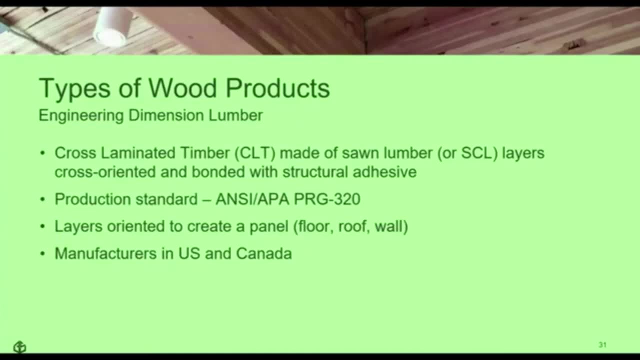 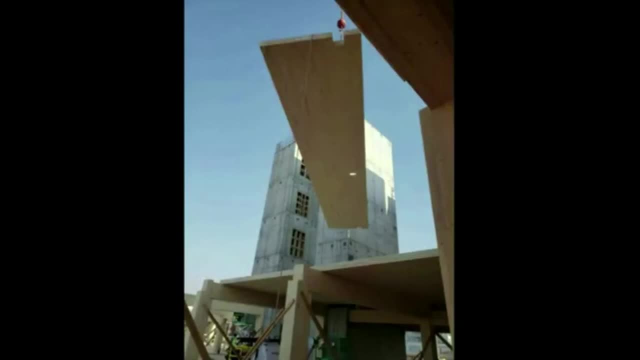 use a European supplier, you need to make sure that that the panels they're producing are produced in accordance with APA PRG 320. so here's an illustration of a of a CLT floor panel being lowered into place. uh, this is a a building in Charlottesville, Virginia, the Apex Energy headquarters. 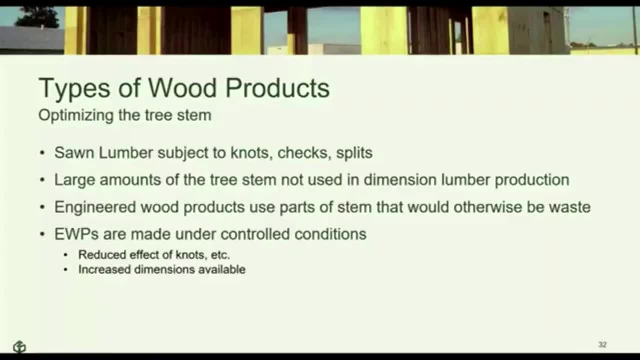 building that was completed last year Gives an accurate description of what's in bride De Bisque. Here is an illustration of that was completed last year. so we've talked about a lot with solid sawn, uh lumber, but what happens with the, the smaller stuff? uh, you know, we have things like knots and checks and splits that. 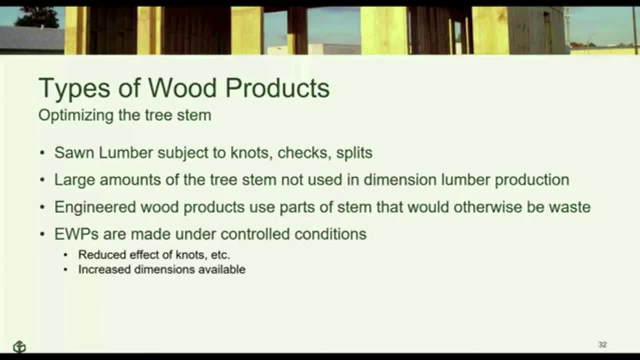 that can cause a degradation in strength of a solid sawn cross-section. we have large amounts of the tree stem that would be not used in the production of dimension lumber, so we don't want to waste that. but what? what can we do? well, we can make an engineered wood product that used 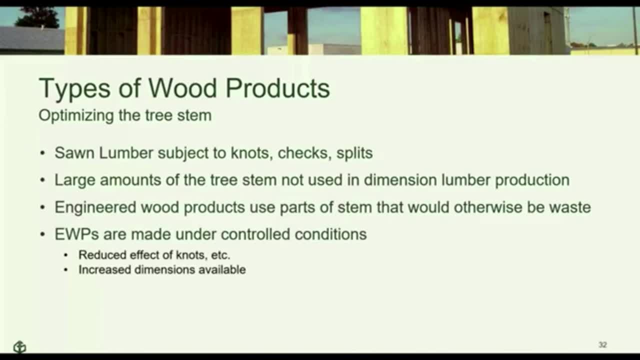 parts of the stem with other that would otherwise be waste, and they also have the benefit of reducing the effects of knots and we can create increased dimensions. uh, so you know it's pretty hard to get a a 16 inch deep board out of a 14 inch diameter tree, but with engineered wood products we actually can do stuff like that. 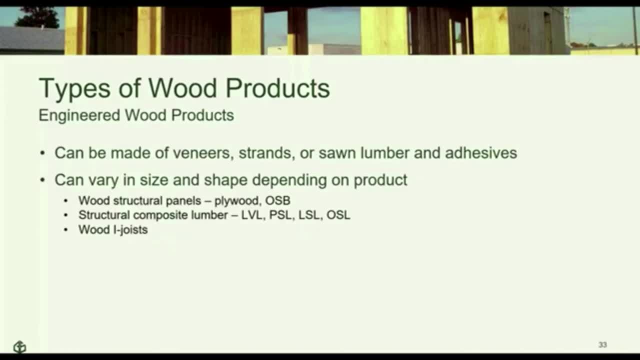 so we can make engineered wood products out of veneers, strands, uh sawn lumber or uh and adhesives, and these products can vary in size and shape depending on what the product is and and what it's and use is going to be. so we have wood structural panels like plywood, and 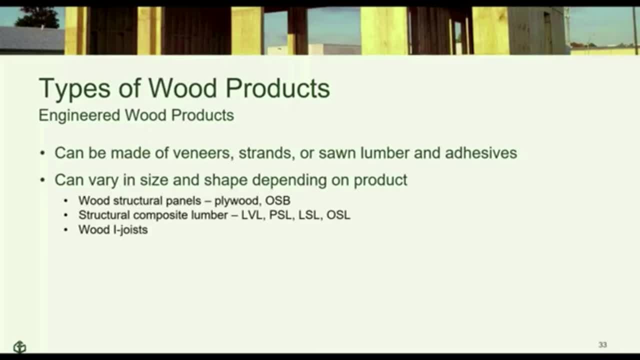 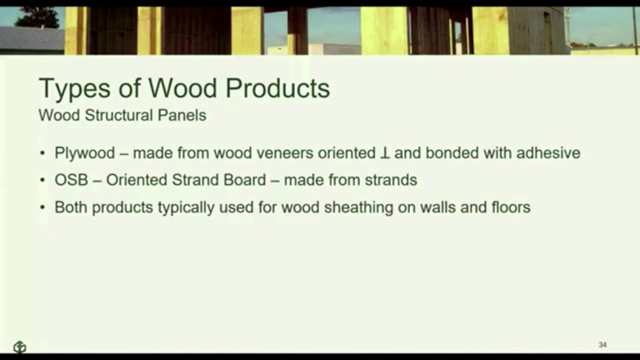 oh, sb. we have structural composite lumber or scl, which i alluded to earlier, and that's things like laminated veneer lumber, parallel strand lumber, laminated strand lumber and oriented strand lumber, and we also have wood eye joists, which are incredibly efficient cross sections that can span long, long distances. so when we look at wood, structural panels are: 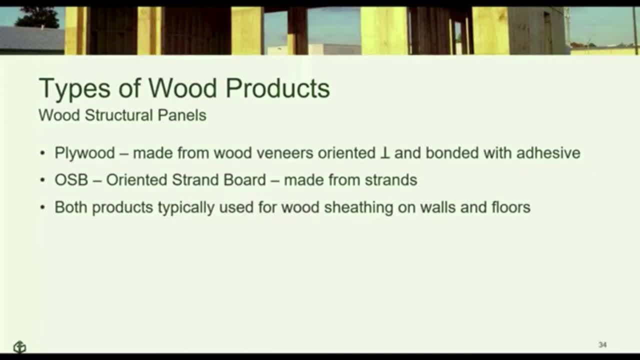 two primary products are plywood, where we use wood veneers that are oriented perpendicular to the adjacent layers and they're bonded with an adhesive. or we use oriented strand board, where we have strands that are actually oriented in a specific direction. it may look somewhat amorphous. 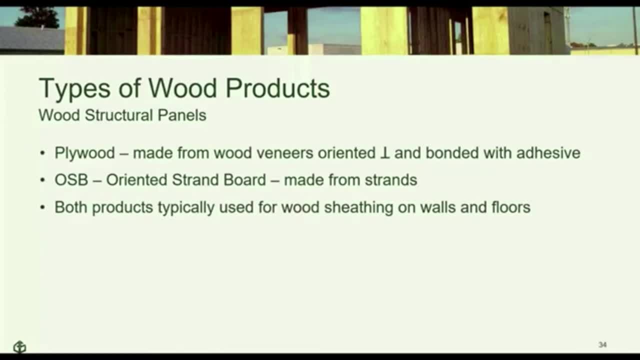 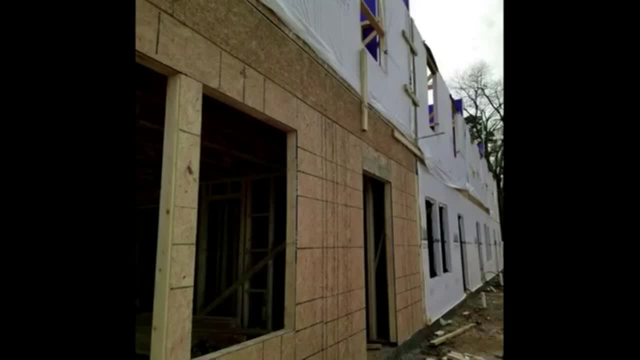 and disarrayed if you're just looking at it, but there there is an orientation of the strands, uh, and these products would be used for for sheets of wood that are oriented in a specific direction. on walls, on floors, uh and, and, as well as roofs, structural composite lumber. 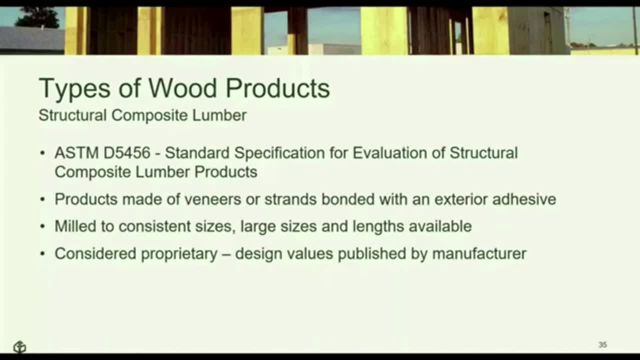 we mentioned are made of either veneers, strands or smaller products bonded with an exterior adhesive. the standard for scl is astm d5456. the cool thing about structural composite lumber is it is a cleaned light steel. then in addition to that, we are also able to use 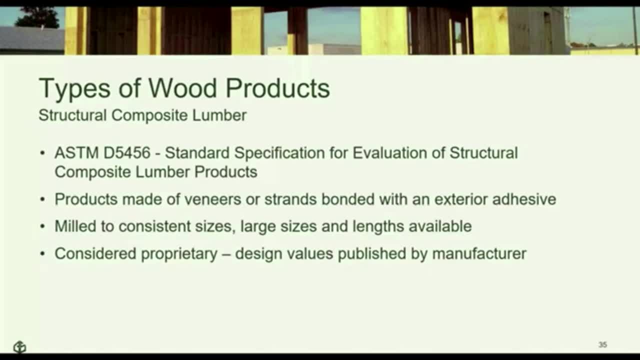 articulated thinking末ニ, looking over on your left hand side, you can see that it's completely different sizes and long lengths available again, because these are being made of smaller pieces of the tree that are glued together, so we're not limited by the size of the tree. These are products that 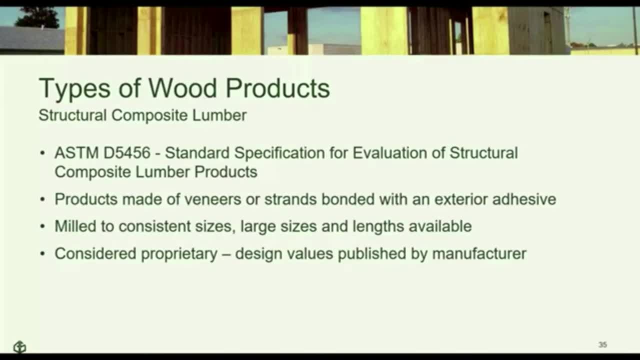 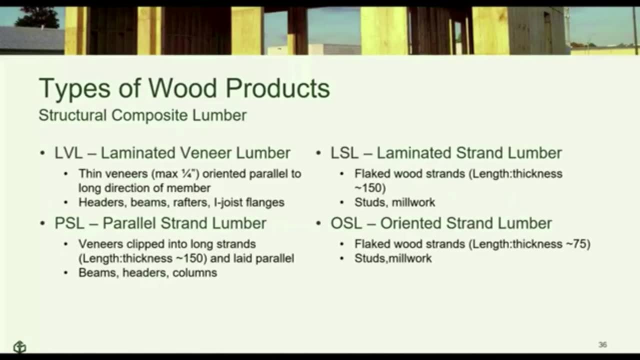 are considered proprietary, so the design values for these products are going to be published by the manufacturer, But these would include, as I've mentioned, LVL, where we've got thin veneers that have a maximum thickness of a quarter inch and they're oriented parallel to the long direction. 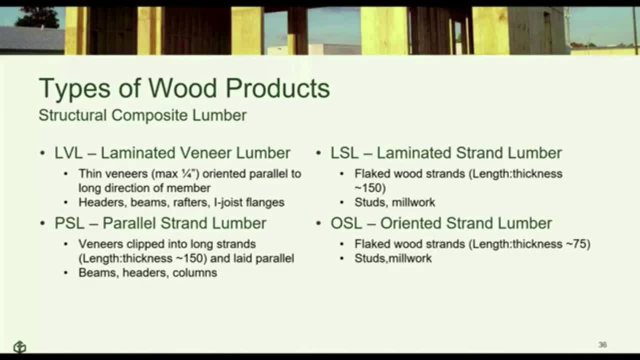 of the member And you see these used a lot for things like headers and beams and rafters, as well as wood eye joist flanges, Parallel strand lumber, laminated strand lumber and oriented strand lumber are all made from long strands where veneers are clipped into long strands and laid either. 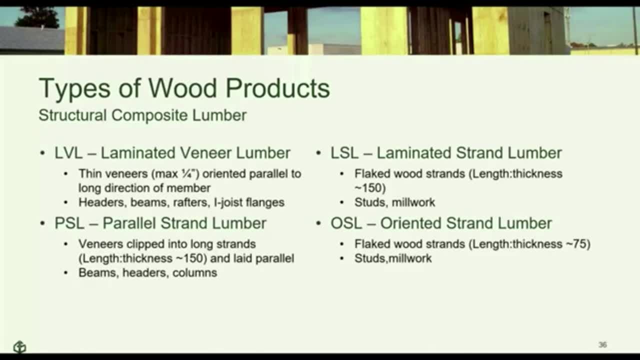 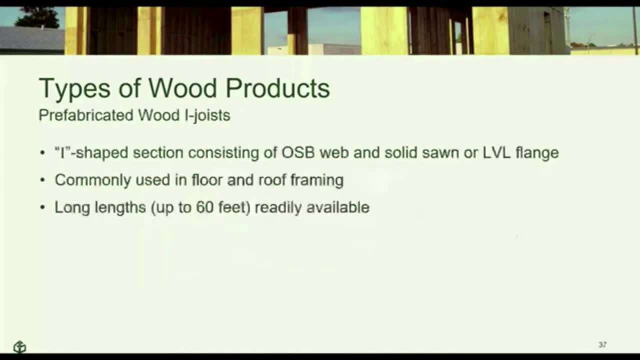 parallel to each other or oriented in a certain direction, And these can be used for various elements throughout a structure as well. Pre-fabricated wood eye joists are shaped like a capital. I so a lot of engineers, are familiar with the eye. 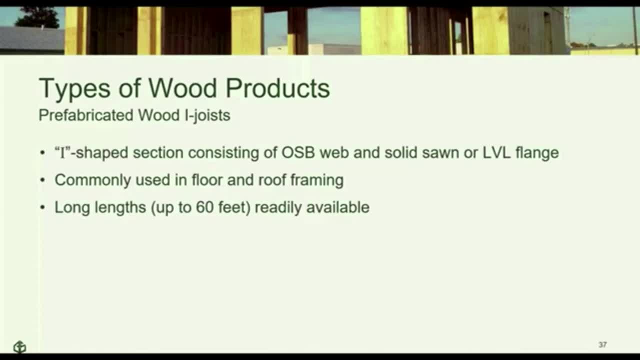 joist shape or the eye beam shape, from steel design, And we all know that the flanges of the eye joists are carrying bending while the web of the eye joist is bending. So if you have any questions, please feel free to reach out to me and I'll be happy to answer any questions you may have. 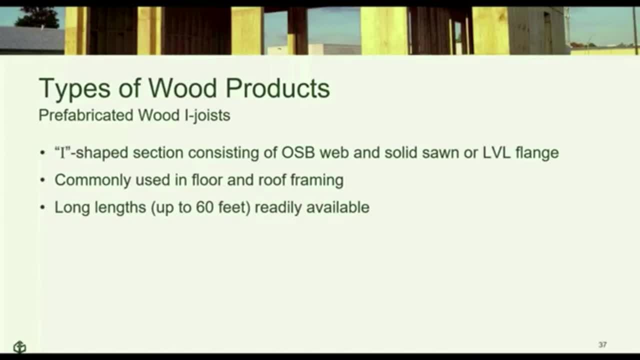 And typically for wood eye joists, we'll see a web made of OSB and flanges made from solid sawn or more commonly- I would say more commonly these days- is LVL or laminated veneer lumber, And we see these used in floor framing and roof framing where you have repetitive framing. 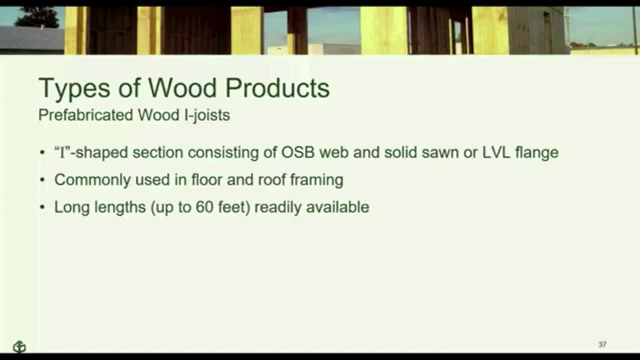 And these can be manufactured in quite long lengths, up to 60 feet- So they can be used for a lot of different things. So if you have any questions, please feel free to reach out to me and I'll be happy to answer any questions you may have. 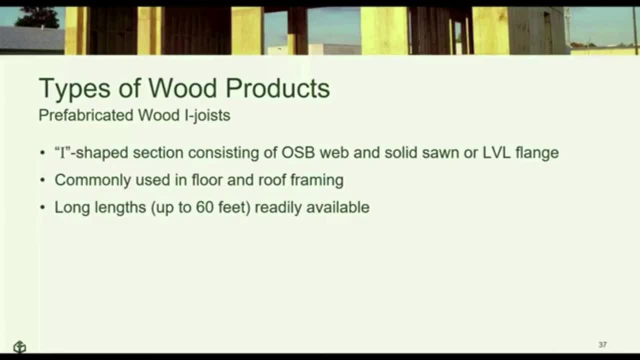 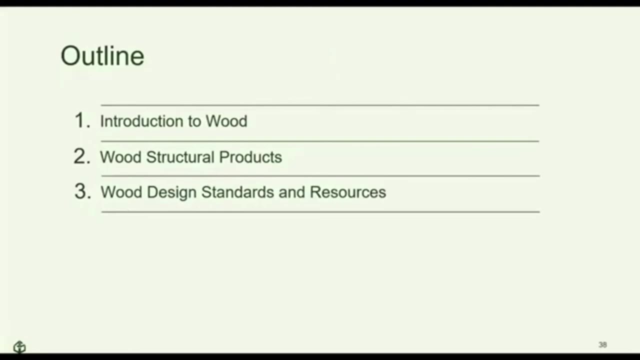 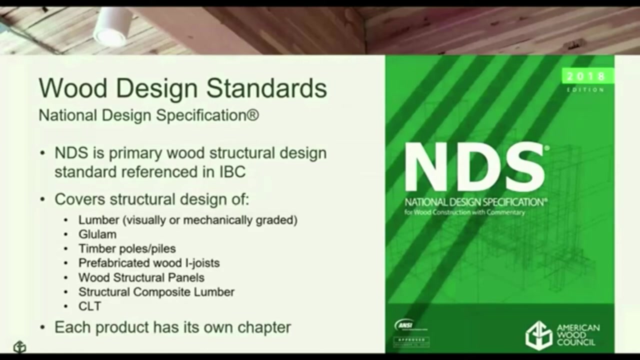 The size options on these is quite extensive and can give you a lot of options for long open spans using wood products. All right, getting into our final portion now, talking about some design standards and resources. So I've already alluded to the NDS multiple times today, so it's only right. 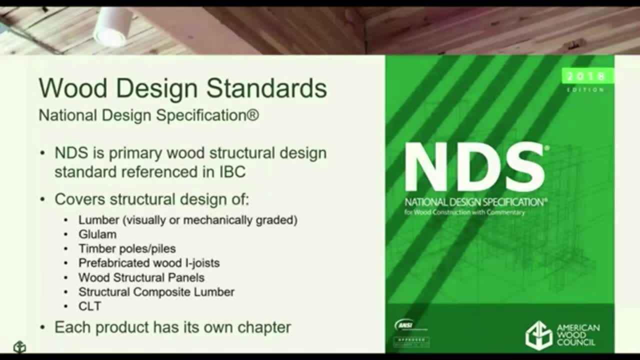 that I give it a proper introduction. The NDS, or National Design Specification, is the primary wood structural design standard referenced in the IBC And it covers the structural design of lumber, glulam, timber poles and piles, wood eye joists, wood structural panels, SCL and cross laminated timber And each. 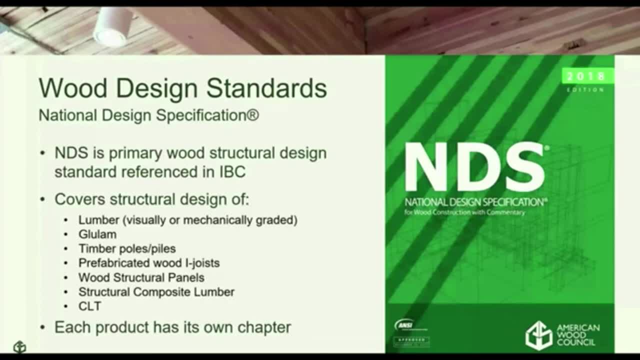 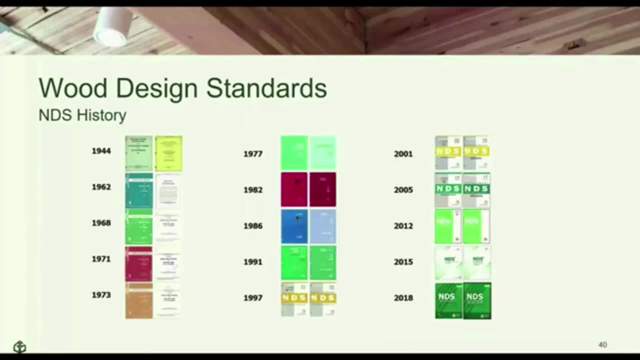 of those products listed there has its own chapter in the NDS. The NDS itself has a long and storied history. It's been around since 1944 and has been updated regularly since then. The latest version is the 2018 NDS. The NDS supplement is an accompanying document. 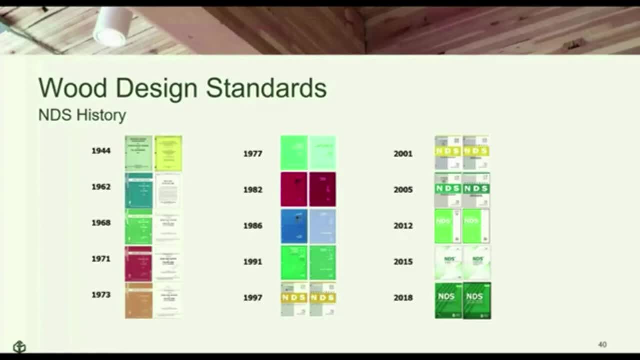 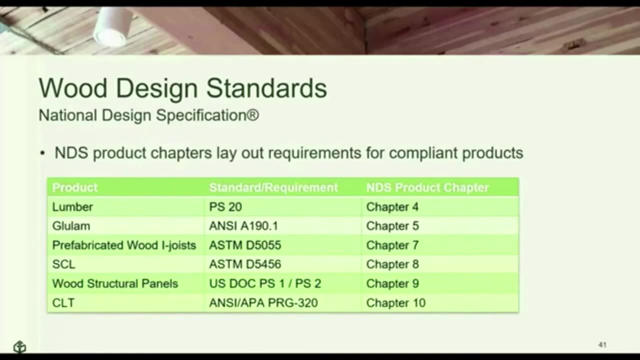 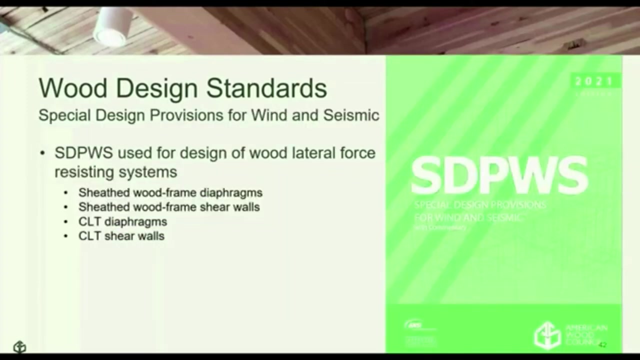 that goes with the NDS. that provides design values for products that are listed in the standard. As I mentioned, we went through most of these standards. When we're dealing with wind and seismic designs, we have a separate standard, the Special Design Provisions for Wind and Seismic, which we affectionately refer to as SPIDWIZ, And this 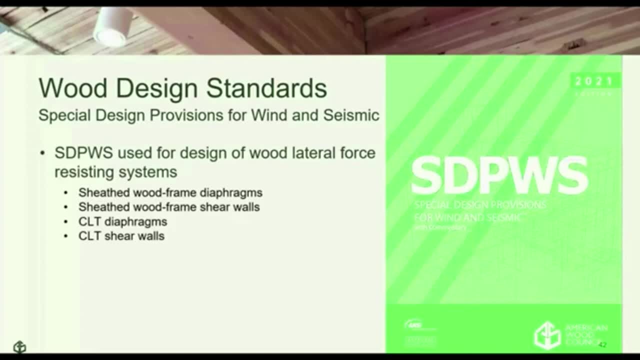 is a document that's used for the design of wood lateral force-resisting systems. The latest version of SPIDWIZ is the 2021 SPIDWIZ. This is the first edition of SPIDWIZ that contains not only provisions for sheath wood frame diaphragms and sheath wood frame shear walls. 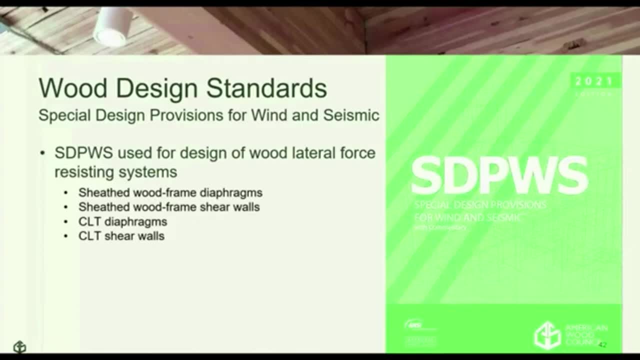 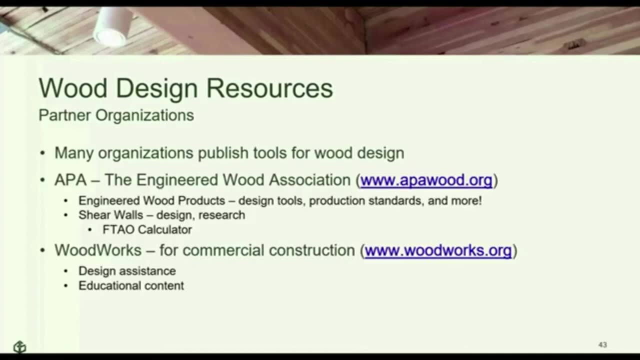 but also CLT diaphragms and CLT shear walls. And then we have some other partner organizations that I would be remiss not to mention as well for some excellent resources, And there's many organizations that publish tools for wood design, suppliers of wood products. So make sure you talk to the manufacturer of 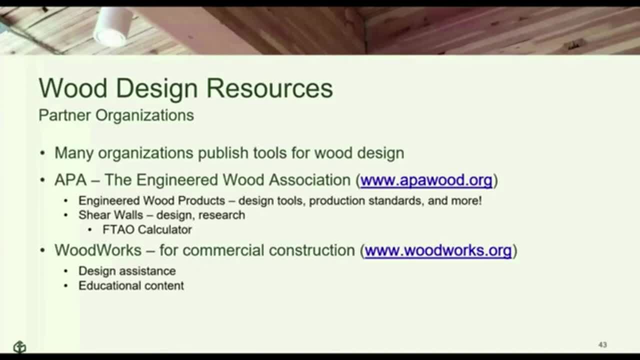 your wood product. They may be able to help you with design tools for whatever type of product you're specifying. So the APA and the Engineered Wood Association has a lot of great information on engineered wood products. They have a really great FTAO calculator for shear wall design. Our friends. 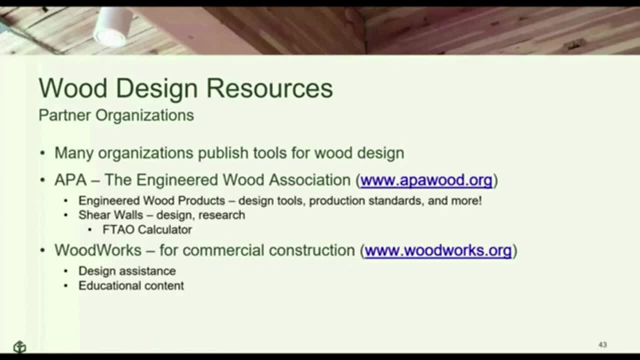 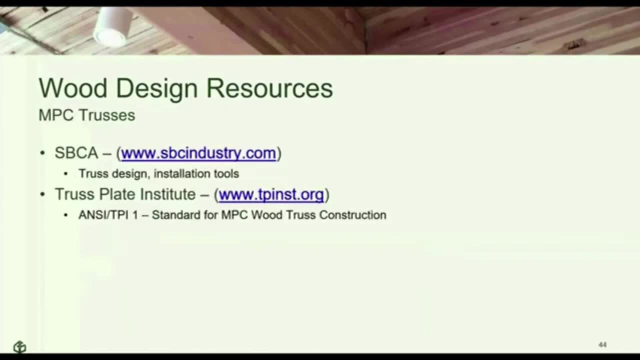 at Wood Works for commercial construction. they have design assistance as well as a bunch of educational content that's really helpful and top notch. I alluded to SBCA for for resources on metal plate connected trusses, as well as the Truss Plate Institute, So here's their. 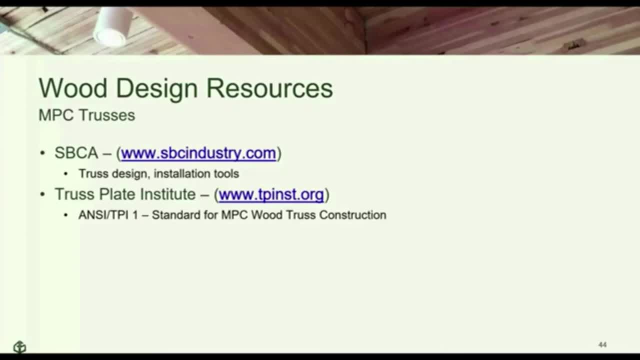 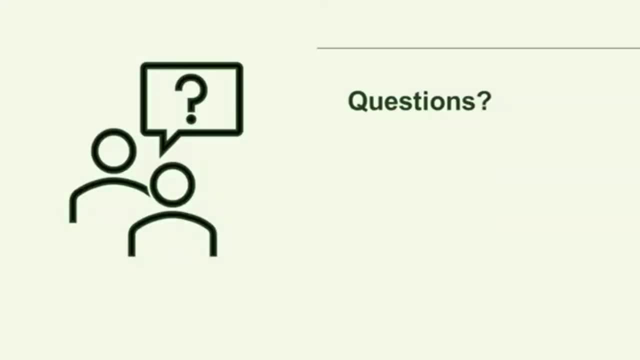 information. You can also find these links in the resources document in the handout section of your dashboard, And with that we'll go ahead and take our questions. Laura Wetzel, TED Talks Office. All right, we're gonna switch over to Lorie for questions. 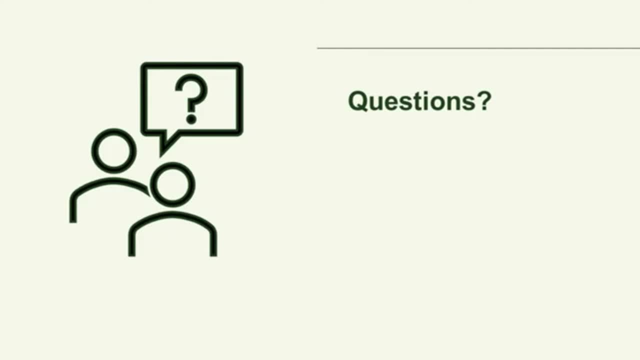 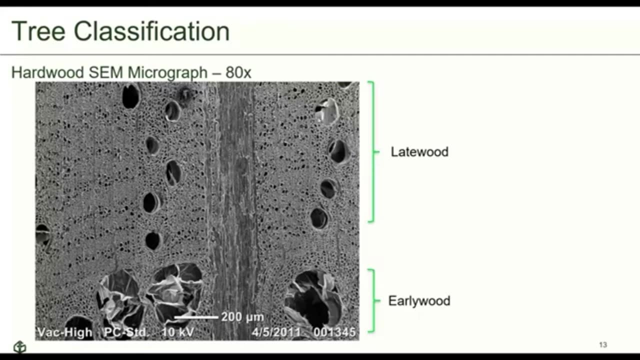 Laura Wetzel TED Talks. Office Sounds good, Laura Wetzel TED Talks. All right here, So you should be able to see my screen here. We had a question on this hardwood scanning electron microscope micrograph here, So I casually breezed through some of the descriptions on some of these cells. 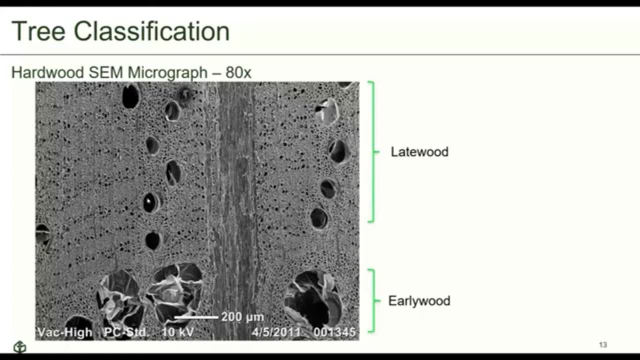 and mentioned the noting which terms stands under theilles at the top. So I asked some of the early wood vessels and late wood vessels which are very noticeable. We see the tracheid cells which are kind of these. you call it the infill if you want cells that make up a good amount of 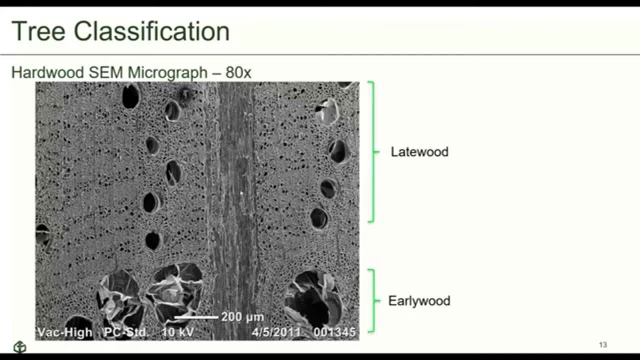 the cross section, But we have this big kind of highway looking fella right down the middle of our picture here And that is actually a ray cell, So we don't see those as nearly as pronounced. They're not common in softwoods but they will be visible much more frequently in hardwood trees. 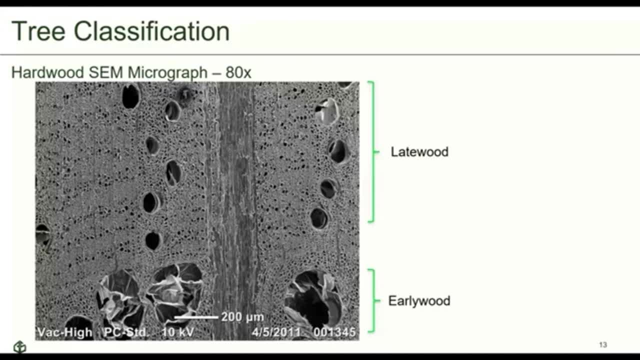 So that's what that photograph that is and those cells are All right. getting into some of your other questions here, All right. what is the moisture content of wood at the fiber saturation point? So, like many things with wood, that varies from species to species And the reason that that particular. 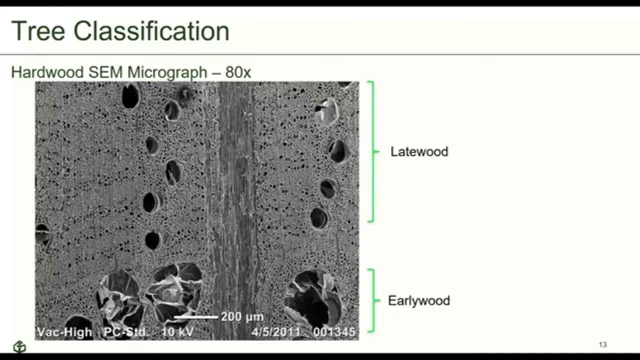 moisture content will vary from species to species depends on the presence of extractives in the wood. So species that have a low presence of extractives will have a higher moisture content because there's more room for the moisture to hang out in the cell walls. 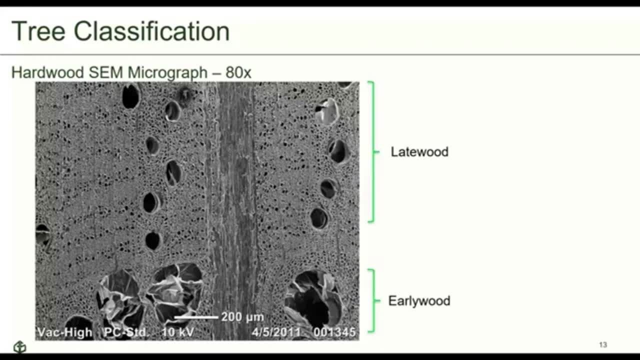 But species that have a higher presence of extractives, like a red cedar for example, will have a lower moisture content at the fiber saturation point. So, like everything else with wood, it kind of just varies with the species. Okay, a question regarding terms and usage. 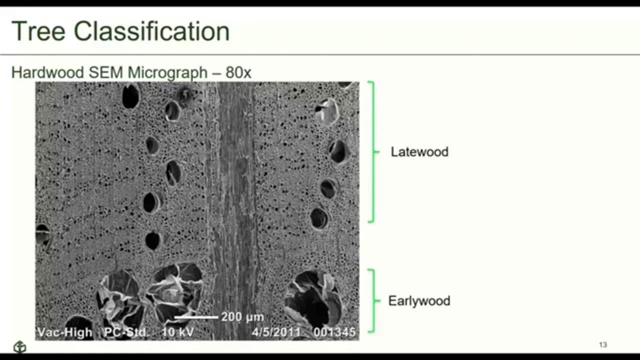 Is CLT the same as mass timber, So mass timber is an umbrella term and it does include CLT. It doesn't include cross-laminated timber, However. it includes other products as well that meet certain size requirements, So mass timber buildings can have glulam elements in them. 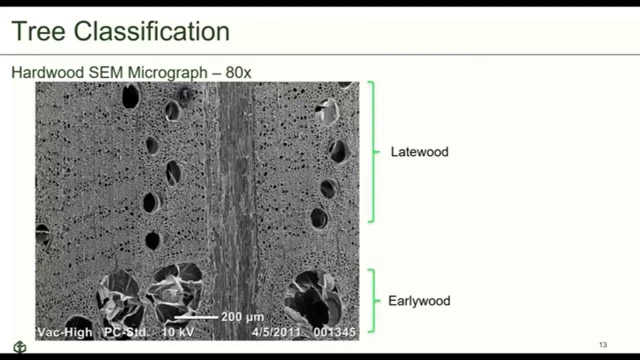 They can have structural composite elements in them. All you need to do is, you know, verify that they meet the minimum cross-sectional requirements that are in the IBC. Okay, Here's a question. We have our nominal sizes of woods that we talk about. 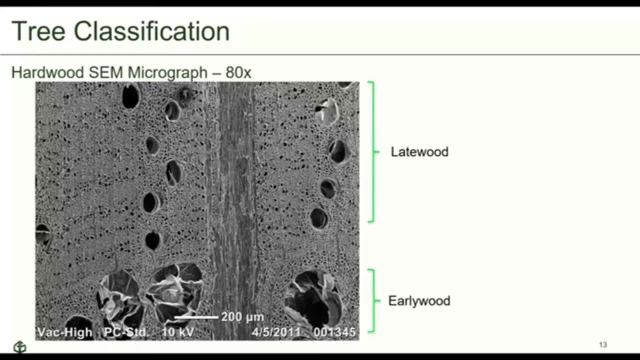 So, for example, 8 by 8 would be an example of a nominal dimension. What are the actual dimensions? If you are in your NDS supplement Table 1B, that provides you with actual dimensions as well as some other geometric and engineering properties that you can use in your calculations. 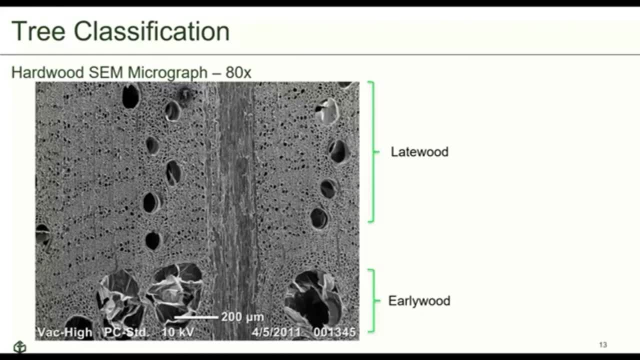 So it gives you things Like the area, the I value, the S value. So if you're not familiar with that table, definitely take a look at it. It's very helpful. Oh wow, You guys have a lot of questions rolling in. 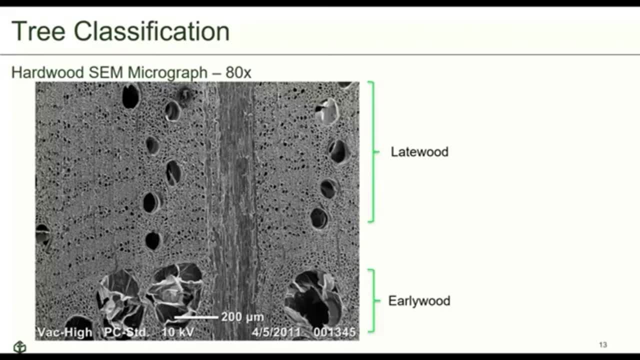 So just give me a moment to read a few of them. Okay, Related to lengths on products like LVLs and wood I-joists. So typically the length will be constrained by the transportation of the product. So I've spoken with folks that work at I-joist manufacturing facilities. 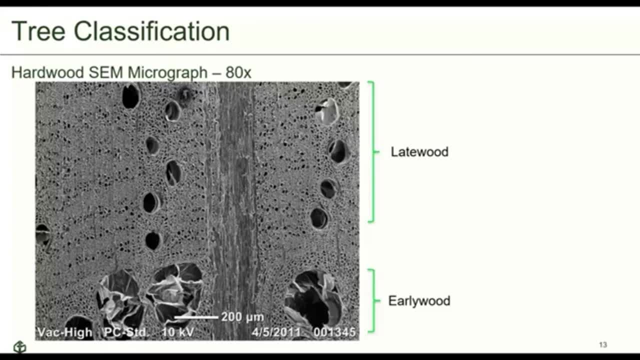 and they can manufacture 60-foot long I-joists And, you know, in certain instances they could even go longer. The challenge becomes transportation of those elements, you know, like any long-span beam. So that is something that you know. these long members are readily available. 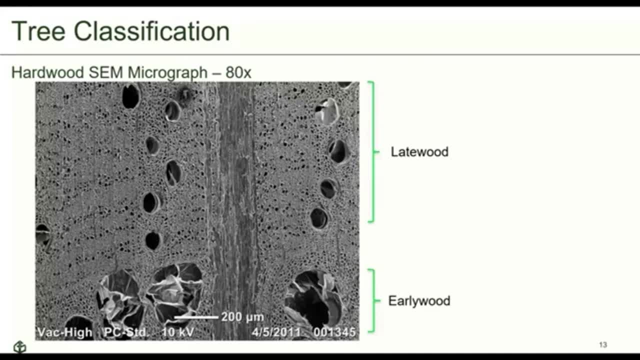 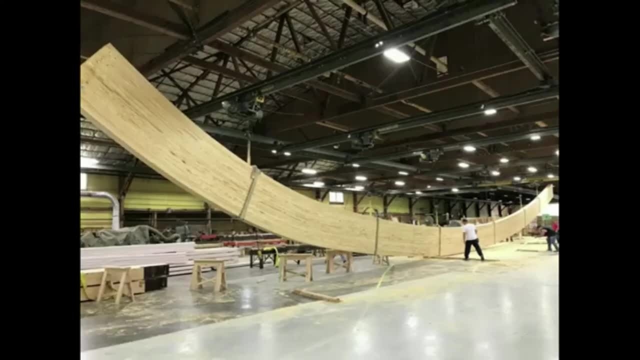 You know, Unilam, we showed you that really lovely custom glulam arch that they had produced. Yeah, We had this really nice custom glulam arch. You know that Unilam has that. they've made glulam members for bridges and other long spans. 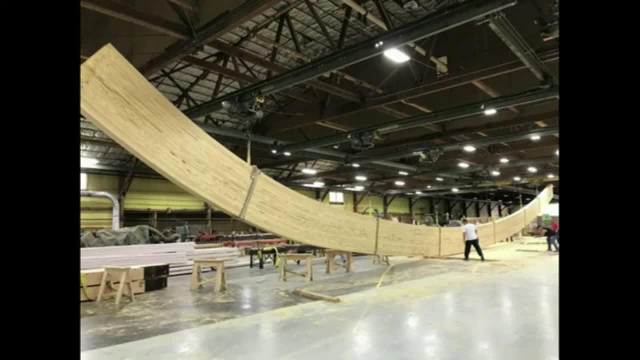 that have been in excess of 100 feet, But you know again they're not that I don't know. The logistics on that come into play and that can be challenging when you're trying to deal with the project management side of elements. 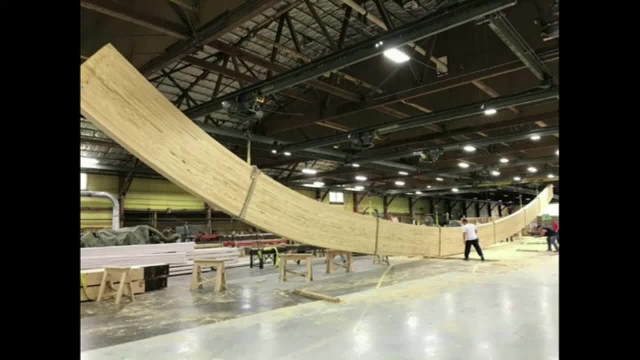 How do they bend the ARCH member that long? I actually do not know the process for creating an ARCH of that size. We maybe can get our folks from UNILAM to come back for a program next year and talk about some of the finer points of glulam construction. 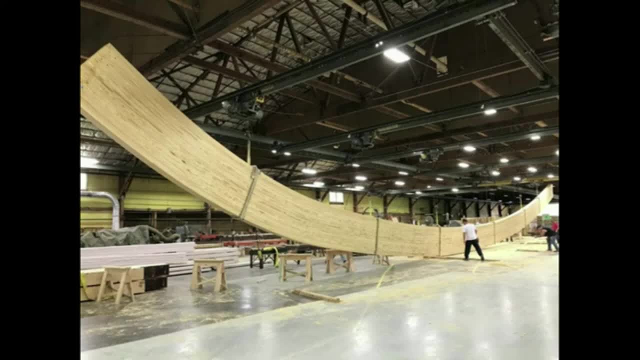 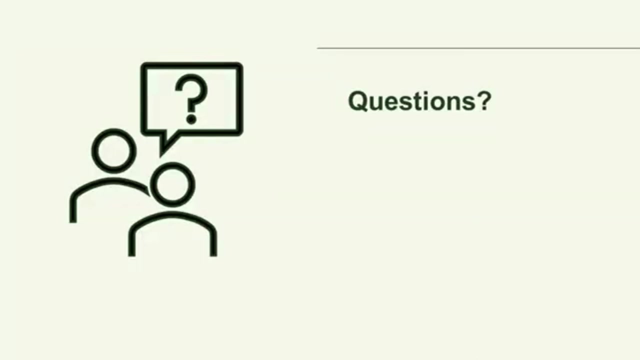 You can also check out our course from last year where we had a discussion panel on glulam construction. What type of adhesives are used for engineered wood? There are various. There are various types of adhesives and it will depend on the product that you're using. 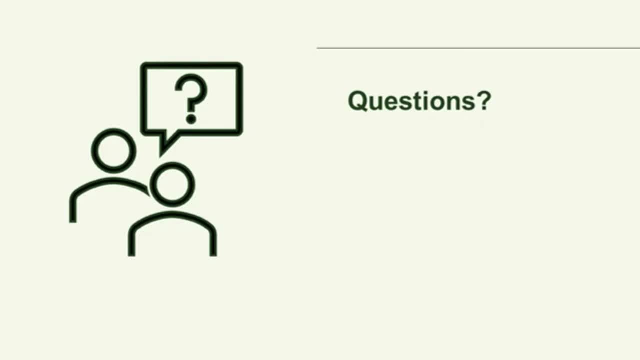 There are some products that are polyurethane-based. There's other products that are phenol-based adhesives. So it just varies with the product, but it will be specified in the production standard for that product what the requirements for the adhesives are. 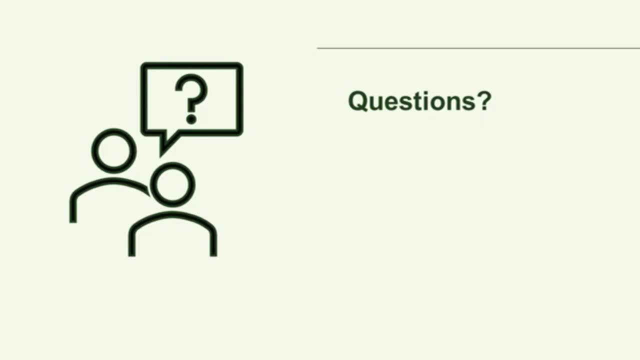 Okay, does the 2021 SPIDWiz include provisions for CLT shear walls and diaphragms? It does actually. We had a great presentation last year by Phil Line on the 2021 SPIDWiz where he talked about some of the updates. 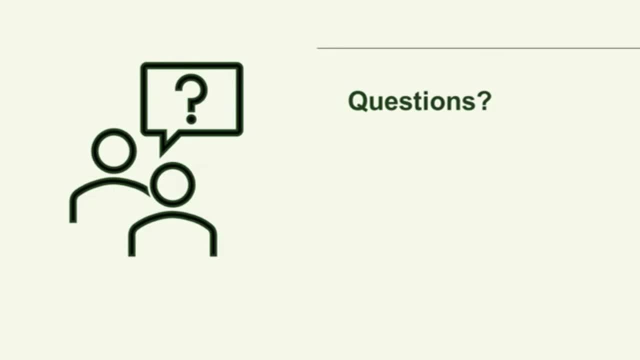 And that was one of the biggest updates was the addition of CLT shear walls and CLT diaphragms in the new version of the special design provisions for wind and seismic. So there are some big options that we have to work on. There is some guidance out there for folks. 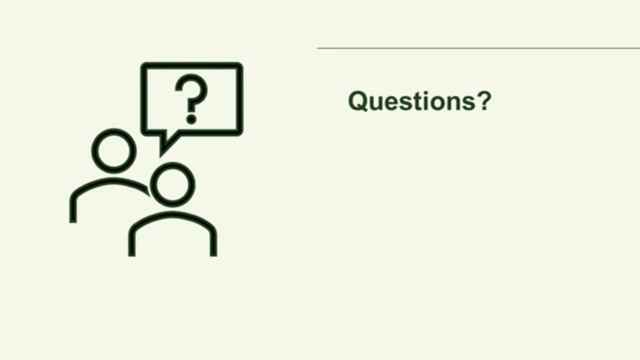 in sections 4.5 and 4.6, as well as Appendix B. Okay, in SPIDWIS. are OSB and plywood considered wood structural panels? Yes, in SPIDWIS, typically when the term wood structural panel is used. 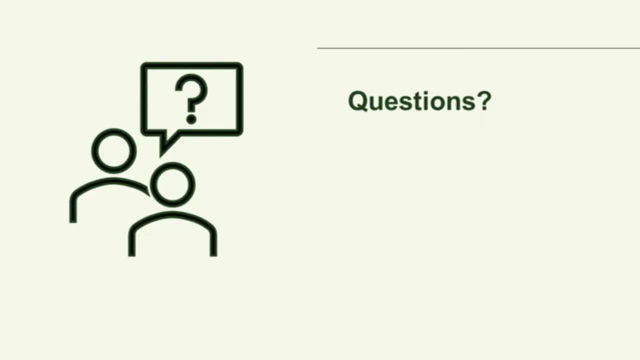 it's referring to an OSB panel or a plywood panel. Okay, here's a great question: How does pressure treating affect the moisture content for design stress purposes? So typically when we have pressure treated lumber, it will say on the grade stamp KDAT. 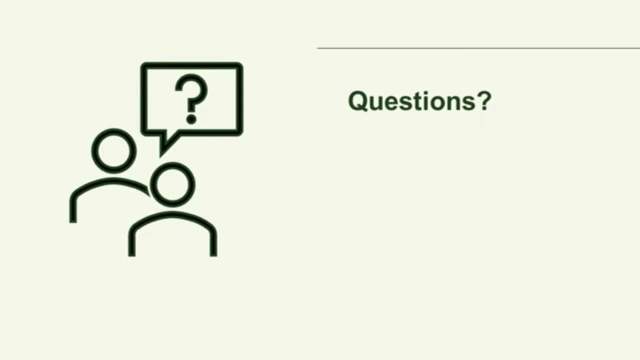 which stands for killin' dried after treatment. So most often the pressure treated lumber will be dried or will be treated, and then it'll be killin' dried So we can treat that lumber as a normal moisture content. We wouldn't have to apply the wet service factor. 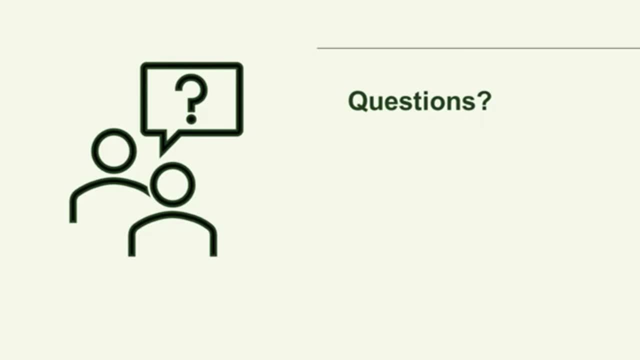 All right. how is salvaged or reclaimed lumber graded? That is, there's the same way that non salvaged or other lumber would be graded. a reclaimed lumber, you, you can get. uh, there are services out there where you know wood grading professional can come to a site and grade lumber and if it needs, you know to have the grade stamp. 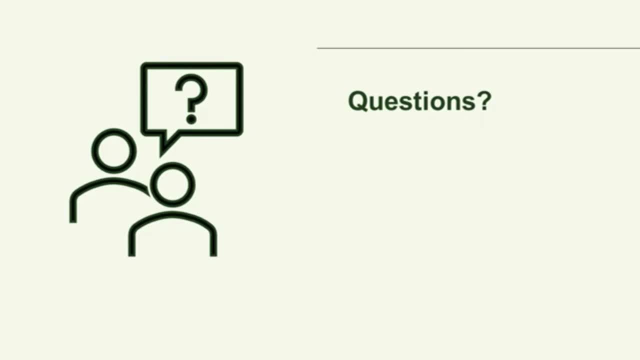 or you know the grade adjusted those services are, are available, um, but but uh, regraded lumber isn't something that we we really specialize in. oh, i've got a great a note here: the the glulam arch in the photo here is 125 feet long. thank you, 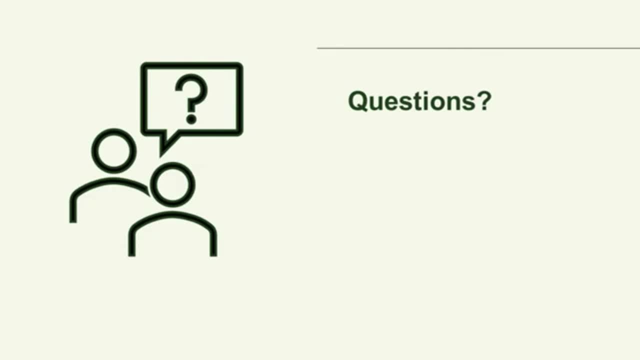 for that that's an excellent figure. so again, very long lengths available, especially with you know, these engineered wood products can be manufactured to you know any size uh that you're, you can imagine, uh, it's just a matter of getting it from where it's being built to your job site. 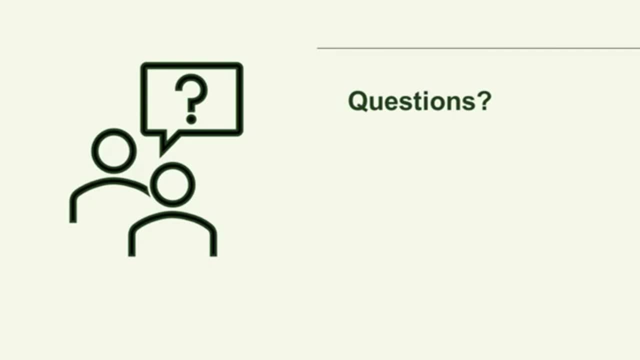 so, all right, how is? here's a couple of questions on fire. how is fire resistance provided to wood? uh, so the we just had a new standard approved, and it's on our website, called the fire design specification, or fds, and that, uh, coupled with nds, chapter 16, give a whole a lot of information on. 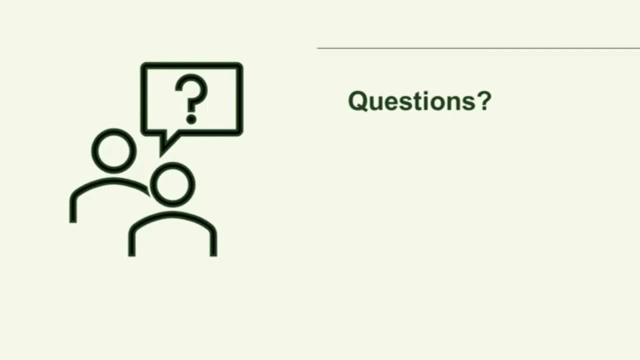 fire design and fire protection of wood elements. so wood does have a codified char rate, and that's what we're going to talk about in a little bit, and then we're going to talk about some of the things that we're going to talk about in a little bit, and then we're going to talk about 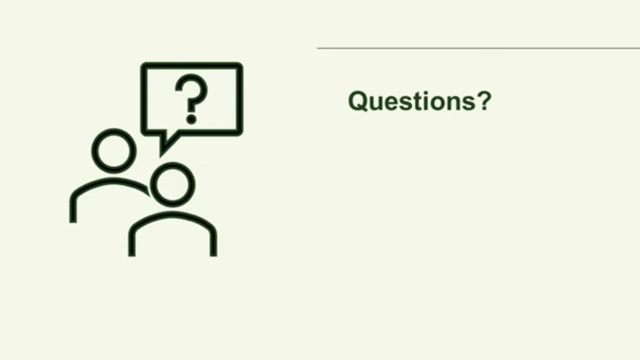 some of the things that we're going to talk about in a little bit, and then we're going to talk about of 1.5 inches per hour. so if your lumber is designed to be exposed, uh, you, you would calculate the required size for your- you know your structural needs- uh, and then you would size the. 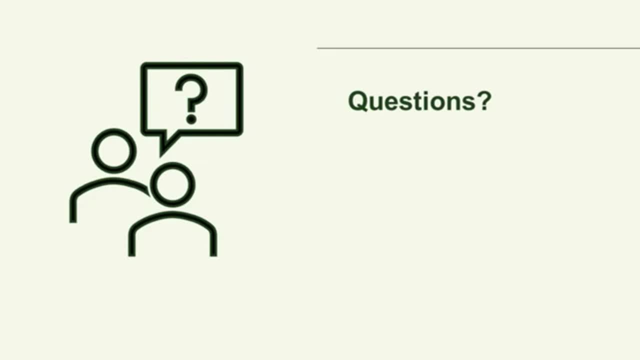 section up, based on how much fire resistance is required and how many sides of the member would be considered to be exposed to fire. so for beams, for example, we consider that a three-sided exposure posts columns would be a four-sided exposure. so you would use the, the uh char rate in chapter 16 and and the provisions. 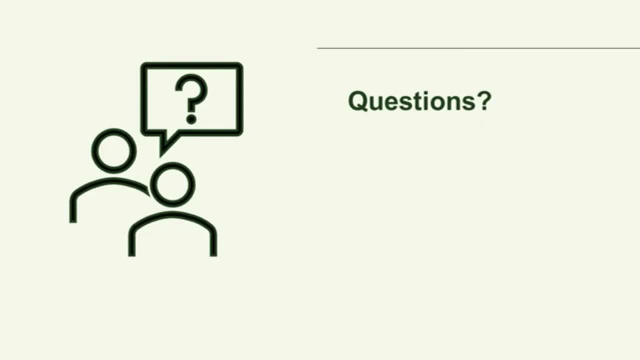 uh, and and that would allow you to provide a fire resistant design uh methodology that is uh acceptable in the in the ibc, in in section uh, i believe chapter seven is the fire chapter. uh, what products are not able to be pressure treated? so, um, oftentimes pressure treatment and gluing are not uh things that can can go together. 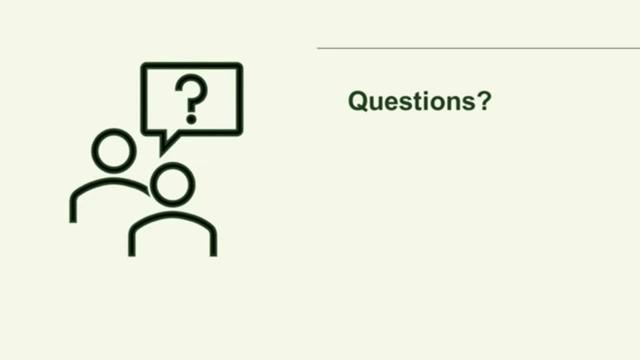 so, um, you'll, you'll need. if you need a pressure treated uh structural composite product or a pressure treated glulam, that's something you'll need to discuss with your, your supplier, to make sure that that is something they can supply, because not all suppliers will have that available.